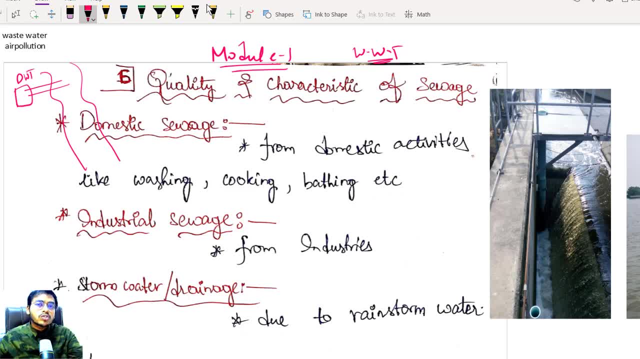 plant. Okay, And this drinking water treatment plant? which code book? it follows IES 10500.. In that, clearly, specifications are given up to what permissible limit you have to treat so that you can supply this water to the people. Agreed So. 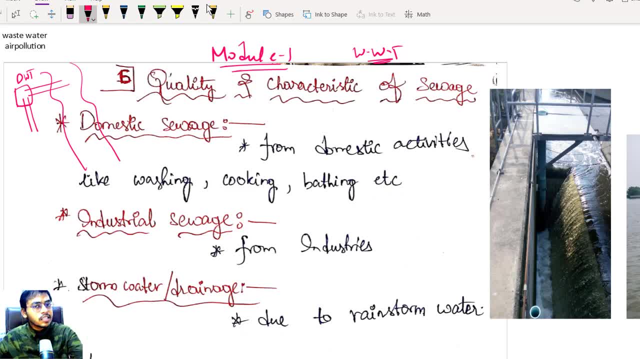 as per IES 10500 or, in some cases, CPHEEO standards, our drinking water treatment plants treat our water and send it to the nearby town. A Okay, Now what is happening to this water? Okay, I have seen a lot of people in the drinking water, even the lower income group people, though gareeb hota hai na. 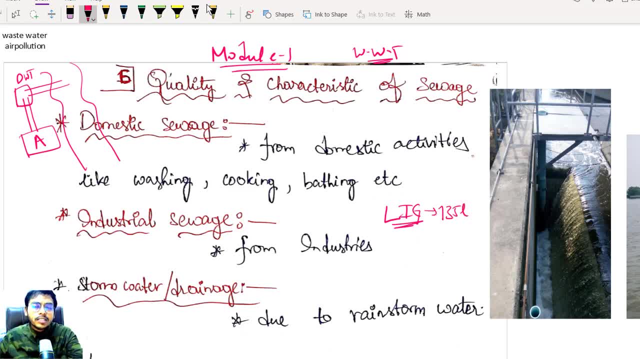 even they consume in India 135 LPCD per capita per day. So every day, each individual is roughly consuming 135 liters in India. What is happening to this water? Okay, Is it a magic? Once you are using it is getting, just it is going out. No right, Where is this water going? Obviously, 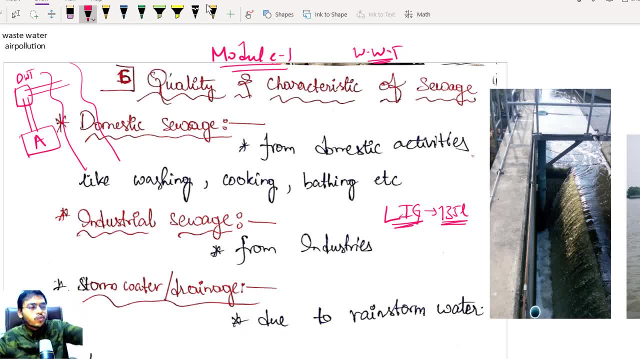 when you are flushing the water, when you are taking the shower or when you are washing vegetables, when you are washing the dishes, when you are washing the dishes, when you are washing the vegetables or clothes, all this water is being sent into our drainage system. Agreed. 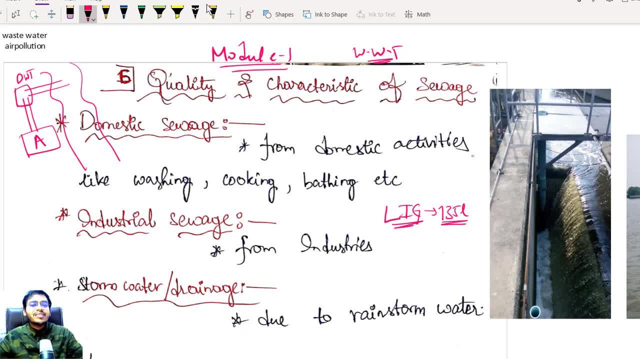 or not? Okay. Into our sewers, Okay. And these sewers take this water to nearby waste water treatment plant. waste water treatment plant: From here we have to treat it again to some permissible standards, Obviously drinking water standards. jitne hai nahi rahega, Okay, We have. 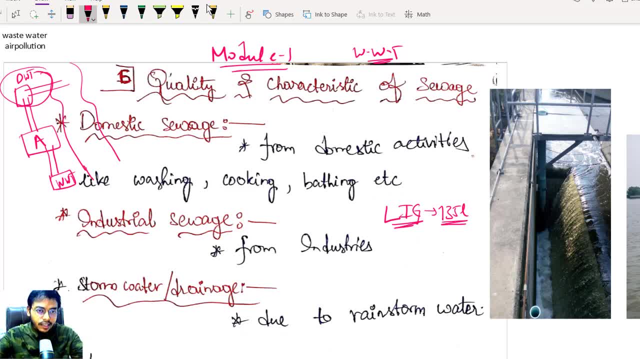 some flexible standards, the standards which are not that strict as drinking water standards, because in drinking water standards we have to consume this water right And we are not consuming this waste water treatment plant directly water right, So the standards are little bit flexible. 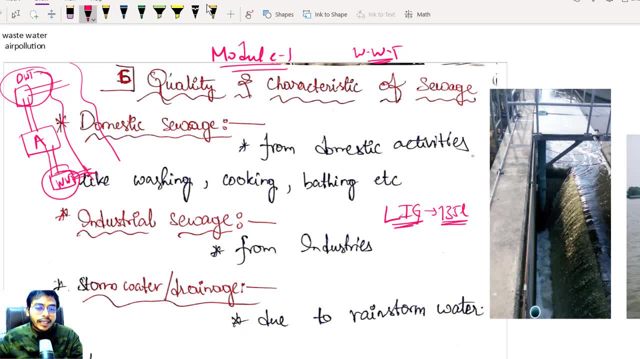 compared to that of drinking water. We treat it and then we send it back into nature, or you can say the same source of water, Okay, This waste water treatment plant is very important. If you don't have it, obviously it might cause a lot of diseases to human beings, not only human beings. 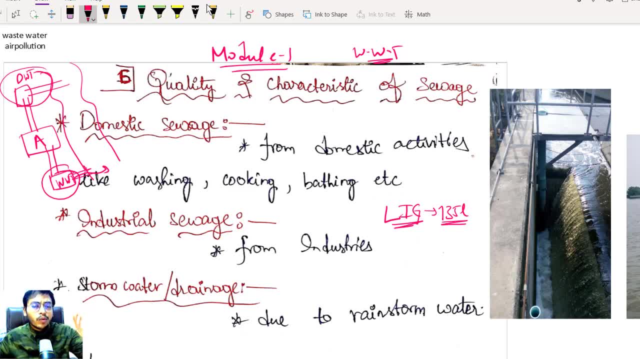 it might cause a huge damage to nature. aquatic life. pura mar ja sakta hai. There is a chance that even entire aquatic life in the nearby region might vanish. I hope you are getting this point right. What is the importance of waste water treatment plant? Now? what is the water which is entering this waste water treatment? plant. Let us try to understand. See, obviously, whatever domestic water was there, it is being collected and sent to your waste water treatment plant In general, in general, 90% of the water, whatever you were consuming, right? 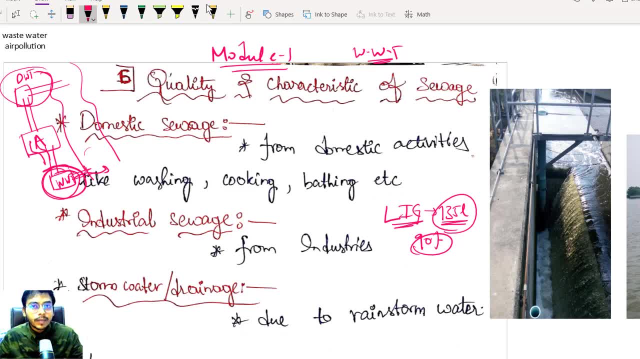 It will be coming back to waste water treatment plant. Okay, It will be coming to waste water treatment plant, Remaining 10%. it will be losses. It will be losses. It might be the percolation losses or it could be the evaporation. 10% will be gone and 90% of the water which you consume. 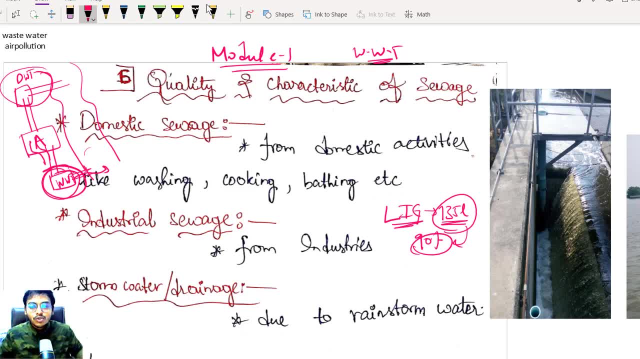 right, It will be going to waste water treatment plant. So far clear, right? So what is the water which is going into waste water treatment plant? Definitely the water from domestic households. Okay, So I am calling this as domestic sewage, The sewage which is coming from domestic activities like washing, cooking, bathing, etc. I am calling 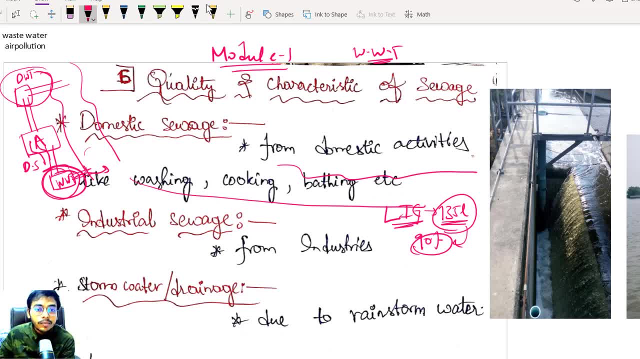 it as domestic sewage. Okay. What else? I will be having some industries agreed. I will be having certain amount of industries, So the water which is coming from these industries is also taken into to our waste water treatment plant. So this water, I am calling it as industrial sewage, Okay. So 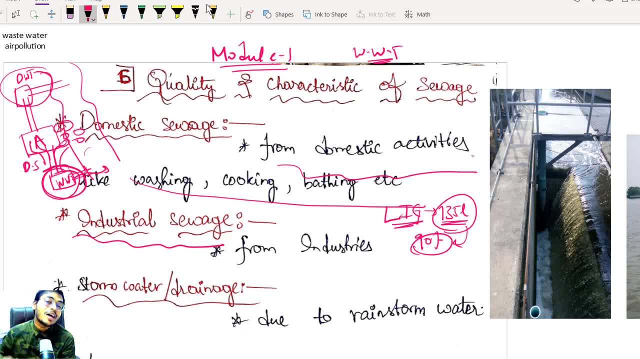 domestic sewage plus industrial sewage. Now there is one more other source. What is that source? See, if in any town, if you have seen, if there is any rainfall, what will happen to this rainwater? Will it stay on roads only? Okay, 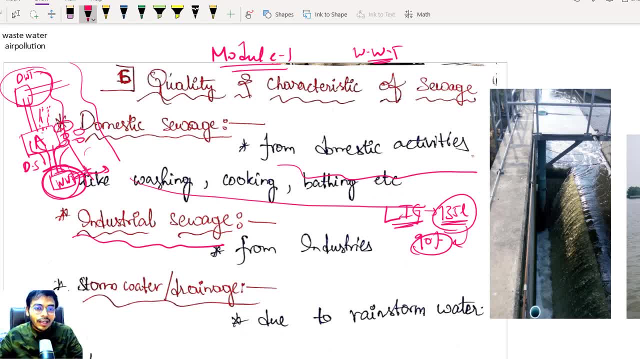 No, right. So the roads will be constructed in a slope, such a way that this water is being collected in the drains and is being carried out. Okay, Agreed or not? So this water which is coming because of the rainfall, we are calling it as storm water or storm water drainage, up to you. 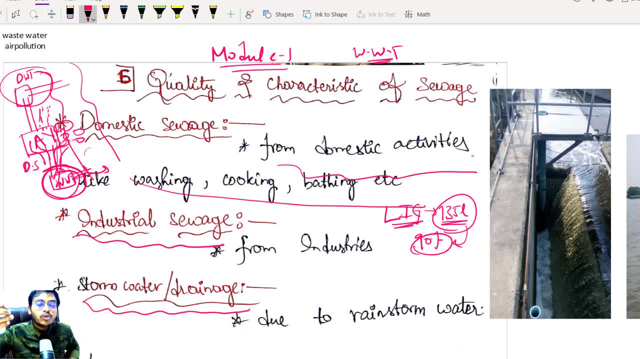 Okay, I hope concept is clear. So what is the input water to the wastewater treatment plant? It is from domestic sewage, industrial sewage and storm water. So far concept is clear. See the water, whichever you are getting in wastewater treatment plant, right, it will be smelly. And this wastewater treatment plant 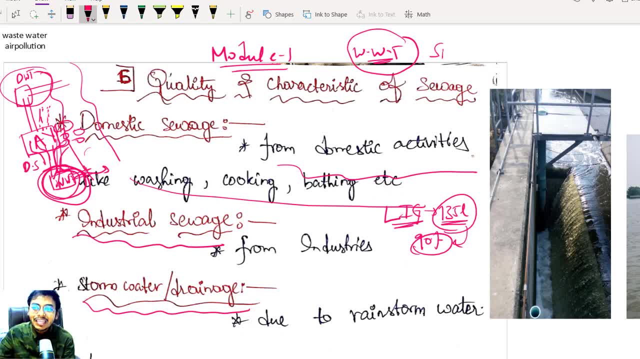 right, it is the smelliest part of our civil engineering. Smelliest, smelliest. you know it right, wastewater treatment plant stinks. Why does it stink? Common sense When you have any organic substance. why do you have organic substance? 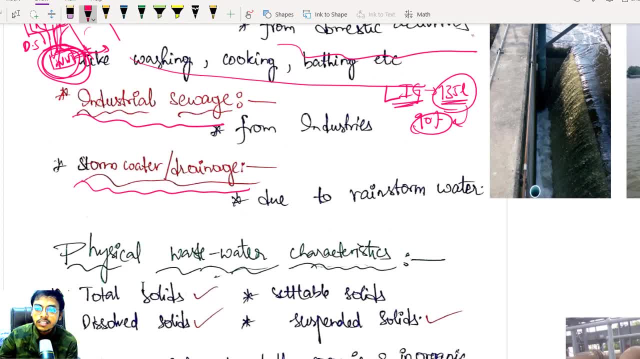 us try to understand, first of all, what is sewage. what is sewage? when i am talking about sewage? right, it is 99.9 percent water itself. okay, 99.9 water itself, but the rest, whatever we have, 0.1 that will be solids, that will be solids. these solids can be organic solids or inorganic solids. 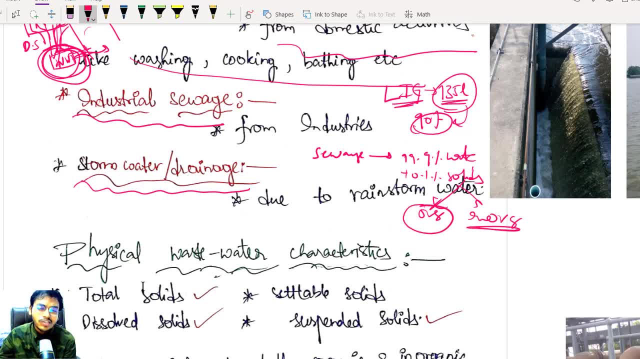 if you have inorganic solids, then not a big deal, but when we have this organic solids, definitely organic solids will be there, right? so these organic solids, what will happen? let us try to understand. if you have any organic substance in nature, what will happen? there will be certain. 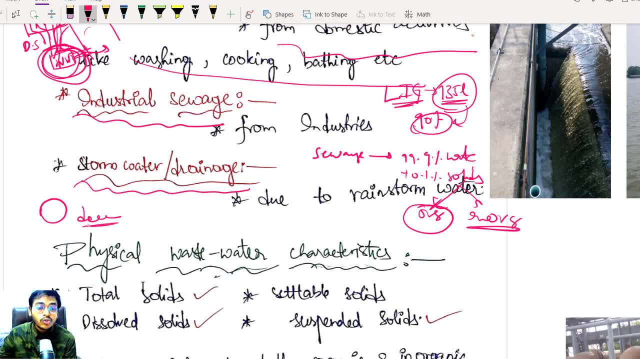 decomposers, which are very active in nature, agree or not, so they will try to decompose it, okay. the same concept is with dead body also right, dead body also decomposes, not only dead body. take some water here and add milk to it, okay. or just take normal milk and keep it outside, just keep it. 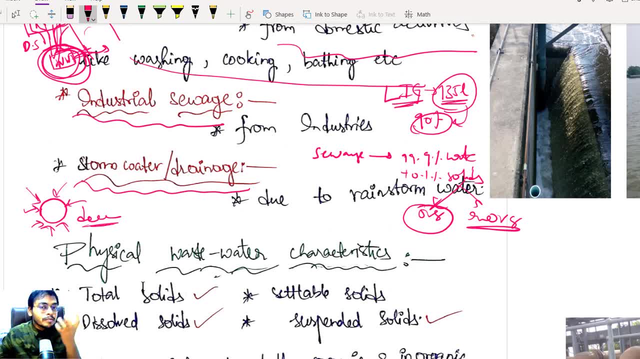 outside your home for two or three days. then go and take the smell. how it will be? it will be very pungent, right, very pungent. why? because the decomposition has already started in that milk. i hope concept is clear why, wherever you have these organic substances, the decomposers will try to decompose it. what are these decomposers? there are some microorganisms in nature which consume their food, which get their food by consuming these organic substances. as simple as that. then why are we getting smell? see, when this organic substance is being consumed by these organic substances, the decomposers will try to decompose it right. so these organic substances are trying to eat this. obviously, there will be some. 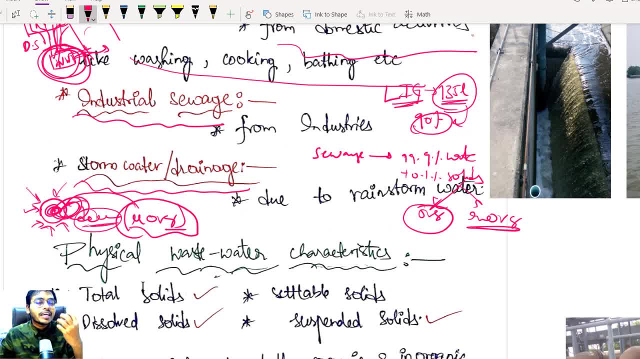 byproducts released right, so that will have sulfur, and not only sulfur. there are many other substances also, but mainly sulfur. so because of it you will be getting that bad smell at the same time. this sulfur is the reason why you will be having this water grayish if you ever see a wastewater. 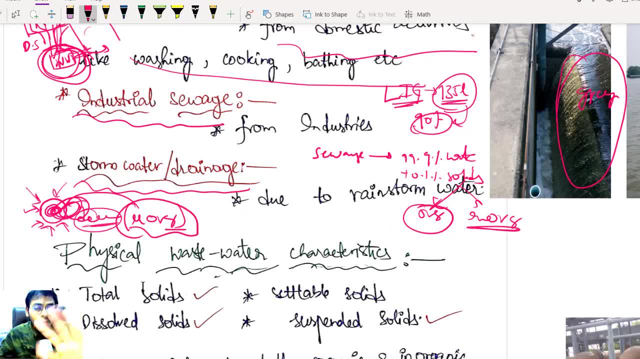 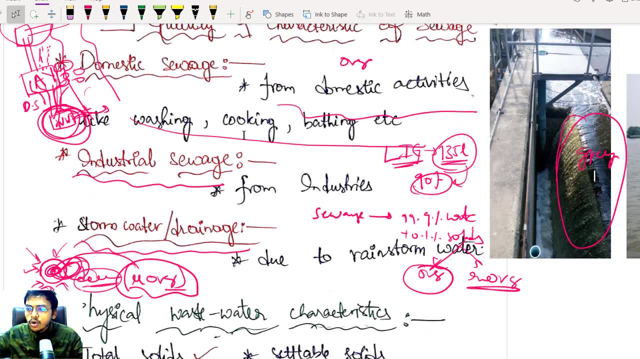 treatment plant water. it will be little grayish, right, i've not drained with a cleaner up, not color of our drinking water, agreed, okay, it is mainly because of sulfur and also other byproducts. now let us try to understand what is happening. or in our wastewater treatment plant, see 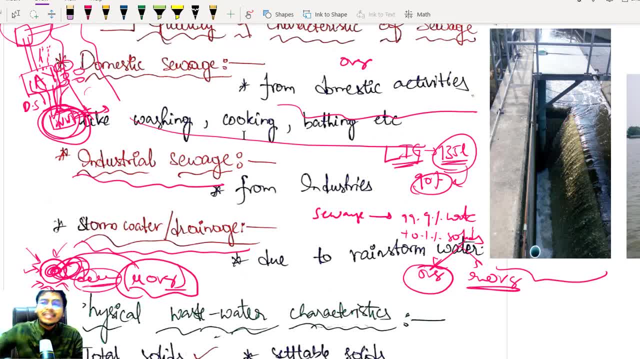 i have taken this photo, my own. i have taken this photo. this is the entrance of wastewater treatment plant. okay, entrance of our wastewater treatment plant. the water from here is being taken to a screening chamber screening, the same screening which we have studied in our drinking water. the layout of our drinking water and wastewater will be very much similar, okay, but there are some. 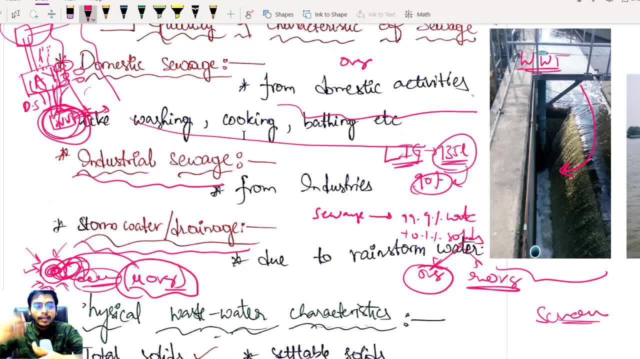 extra things added in our wastewater treatment plant, like great chamber, secondary sedimentation tank and even anaerobic disaster in some cases. we will study in detail- chapter of a coffee, but i are details. but this is how the water looks like. okay, can you see how grayish it is? okay, 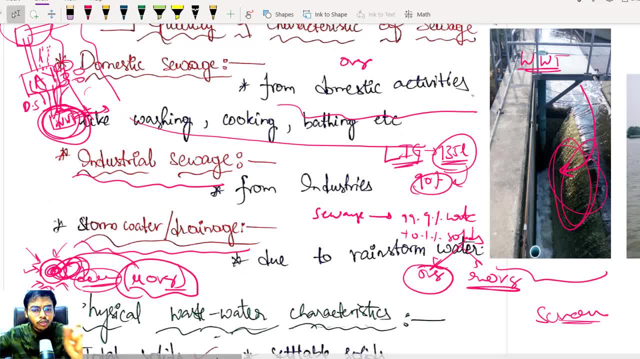 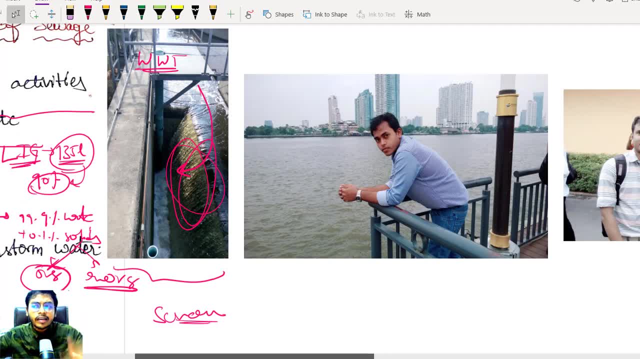 it is very much grayish to dark, black, okay, black to grayish color color: okay, and i have visited a lot of wastewater treatment plants in india and even abroad- okay, so i have visited so many countries. you might be already knowing that i am an environmental engineer. 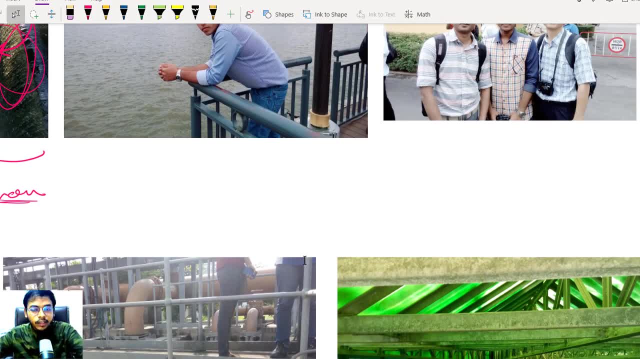 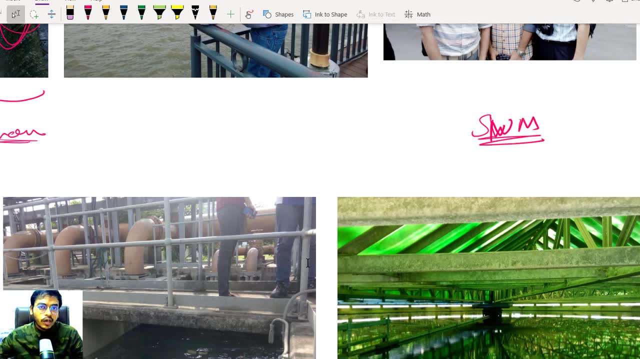 okay, my bachelor's is civil engineering, but i have done masters in environmental engineering and i have worked extensively after my graduation. i have worked in solid waste management. okay, so i have worked in solid waste manager for six months. i have told you this is the smelliest part of civil engineering, right? 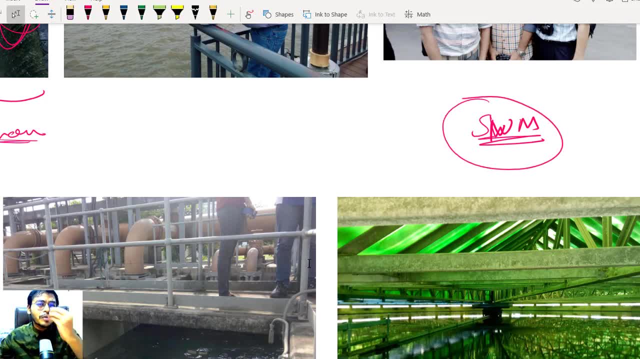 that's the smelliest part of civil engineering, the smell which you get in solid waste management plants. right, you cannot get it anywhere else, you have to experience it, okay, so itna badbu atai, three times, four times water without haloc herramient, and even then it will not go bad with skin. really, the people who work in our solid waste management. 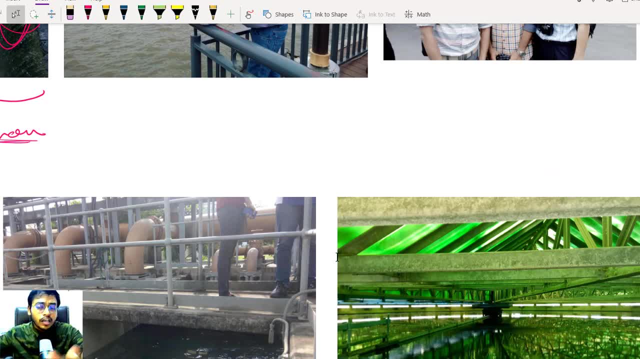 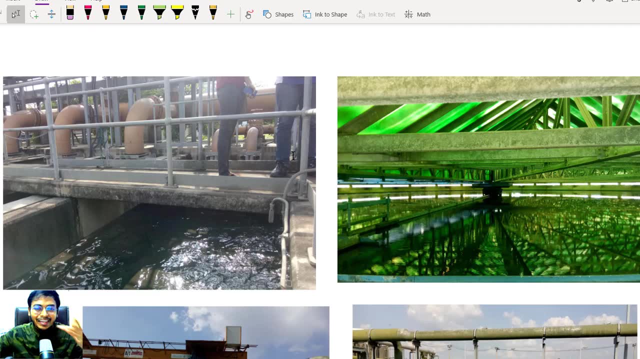 programs. right, sell you to them. i will show you pictures how the solid waste programs looks like. okay, but this is how a wastewater treatment plant looks like. okay, this is some somewhere in singapore, if i am not wrong. so this is how wastewater treatment plant looks like. i have taken this photo. the water is coming inside. you can see how grayish it is, and this: 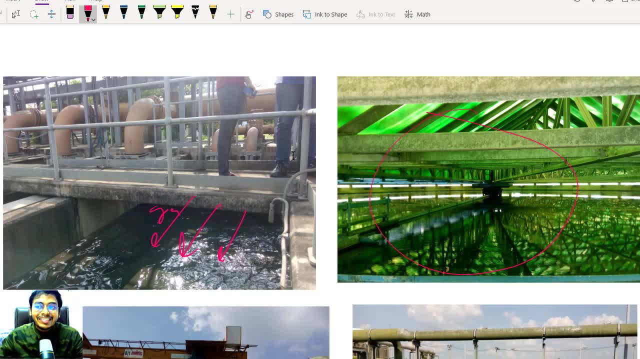 green color. which fancies are the kind of good fancies are the kind of: this is nothing but settling chamber. okay, this is nothing but settling chamber. actually, it has green roof. that's why, because of the sunlight, whatever you are getting, what you are seeing right, it is in green color. 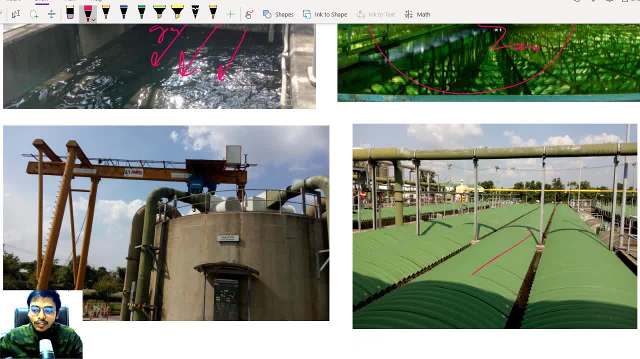 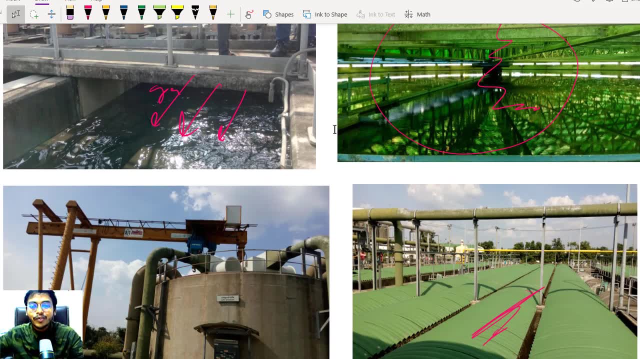 but actually it will be in grayish color itself. okay, so it had some roofs like this. so what happened? the water is looking little bit green here, but actually it will be grayish only. okay, so i will show more pictures, more videos of wastewater treatment plant. not a big deal. 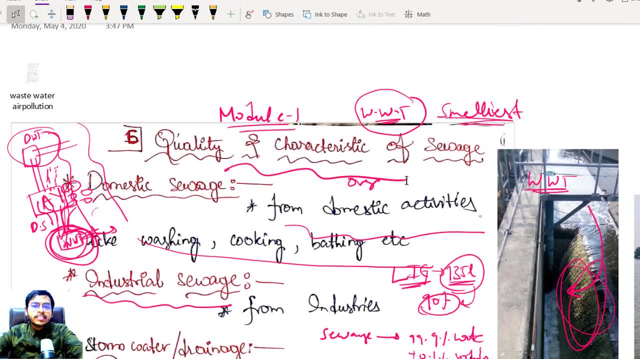 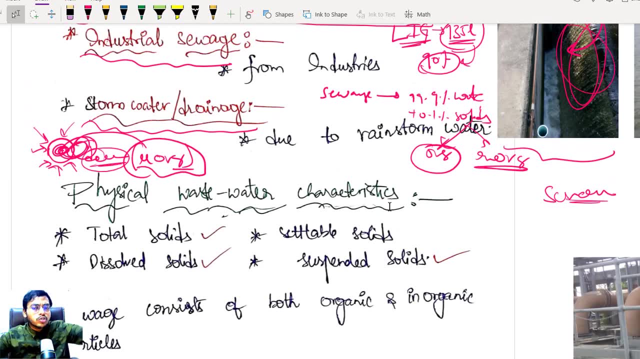 now let us continue with this topic, as the name of chapter suggest: quality and characteristics of seaways. let us see what are the various characteristics of seaway, similar to that of drinking water. we also have physical characteristics, chemical and biological characteristics. let us study them in detail. okay, so first one is physical wastewater characteristics. 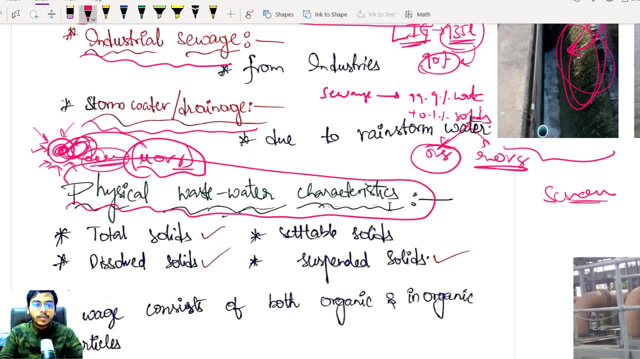 there is absolutely no difference between physical characteristics of drinking water and wastewater. okay, so whatever we studied in that topic- total solids, settleable solids, dissolved solids and suspended solids- see settleable solids. it didn't came in our drinking water, okay so rest. total solids, dissolved solids, suspended solids- the concept is same as drinking. 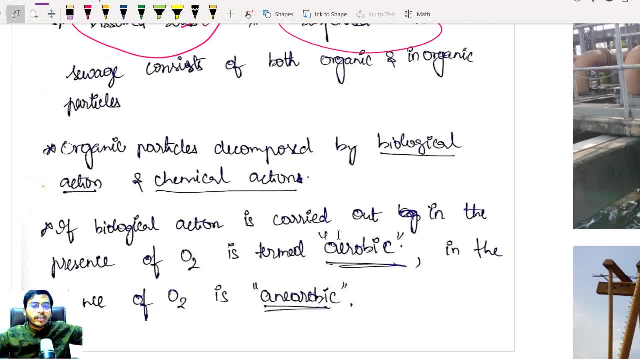 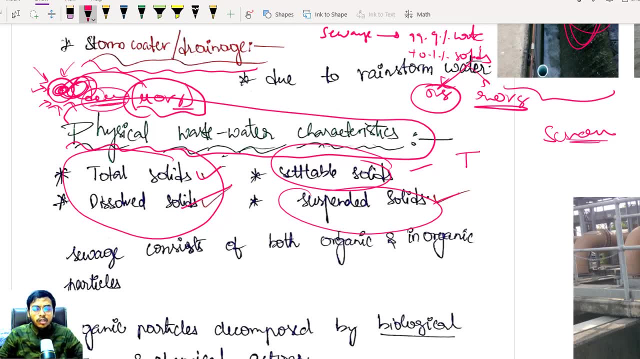 water. let me revise you. okay, i have not given in notes because we have already covered in our topic of drinking water, but let me revise you once. what is this? total solids and suspended water solids- see, basically in drinking water. also there can be this: organic solids and inorganic. 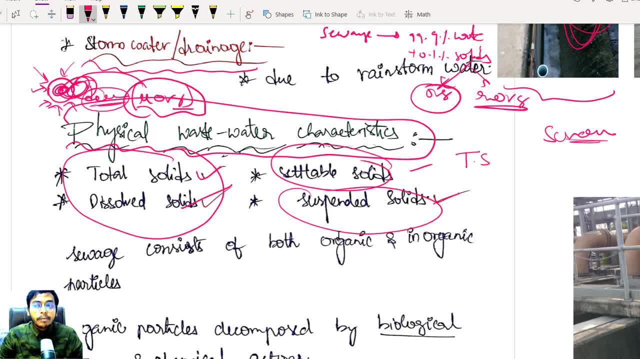 solids in our water right, so we are taking it as total solids based on size. i am classifying this total solids into suspended solids, suspended solids, colloids, colloids and dissolved solids. dissolved solids- suspended solids- are the solids which have the size in the range of 10 to the. 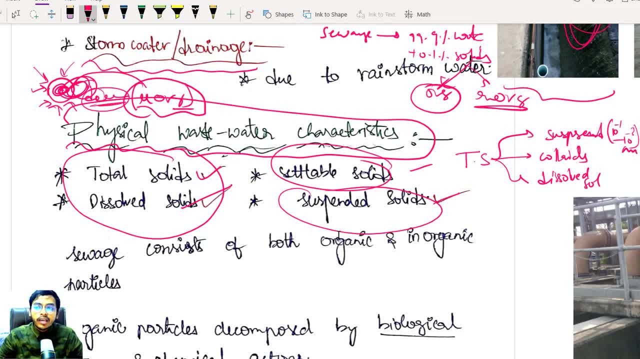 power of minus 1 to 10 to the power of minus 3 mm. okay, so collides are in the range of 10 to the power of minus 3 to 10 to the power of minus 6 mm. okay, and dissolved solids if the size is less than. 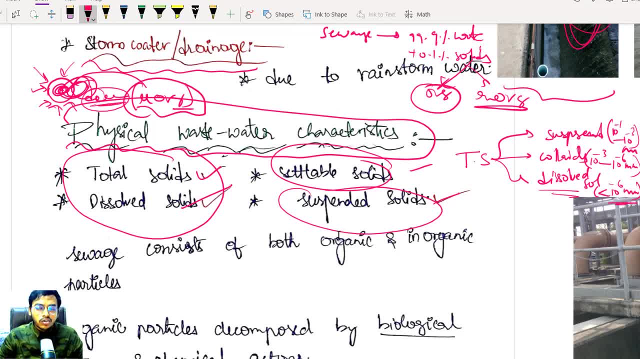 10 to the power of minus 6 mm. we call it as dissolved solids- so small that we are considering it as dissolved in water. okay, i hope you are getting what is? this is all solids, right, and these suspended solids. we call it as non-filterable solids. very important bit. 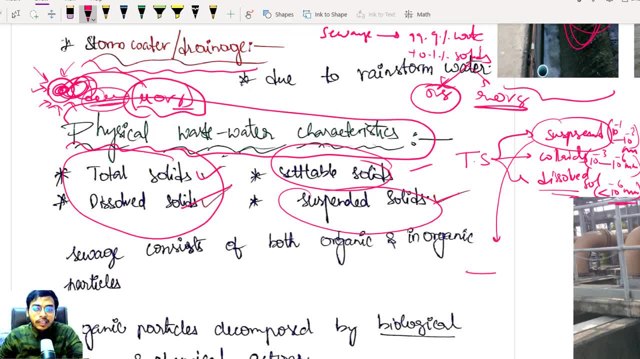 non-filterable, non-filterable and filterable. see, when you are keeping a filter paper, filter paper will be like a very fine mesh, okay. so what is happening when you are, uh, keeping the water, when you are making the water pass through this filter? so what is happening? this suspended solids. right, it will. 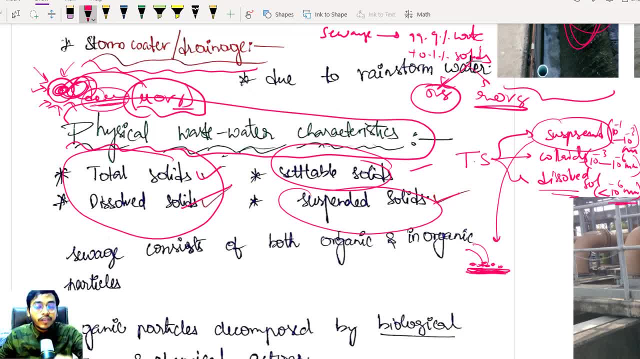 retain on my filter. it is not passing through my filter. that's why it is called as non-filterable solids- non-filterable solids. but this dissolved solids. it will definitely pass through my filter paper. that's why it is called as filterable solids. dissolved solids are filterable solids, okay. 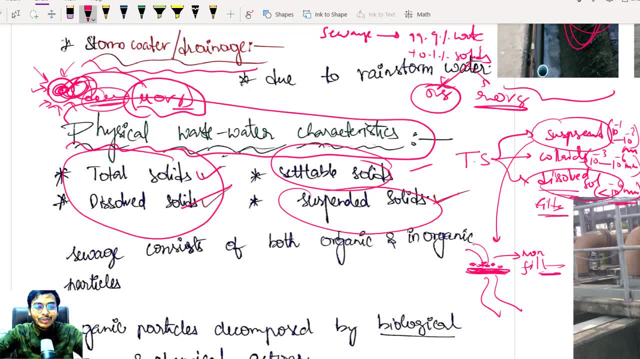 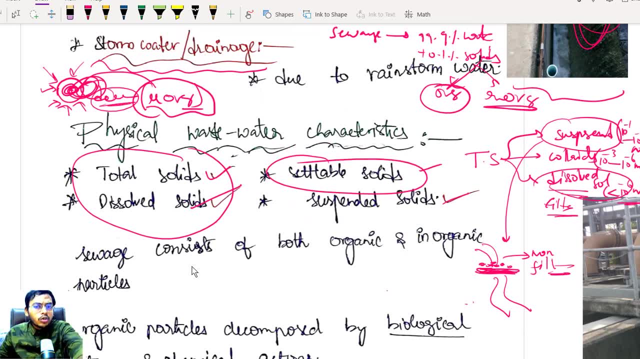 i hope every concept of viewers is reversed. now, related to total solids. i hope you also know how to measure total solids. take certain amount of your waste water, let us say one liter, just for experiment. just for experiment, i am taking one liter of waste water, okay, so what i have, i have. 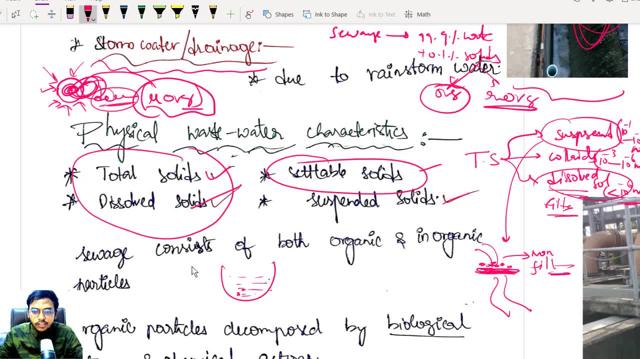 one liter of waste water in this total solids is also present in this total solids is also present in this total solids. so what you have to do, very simple: just heat it to 100 degrees centigrade or, to be present, heat it to 104 degrees centigrade. i hope you remember, in drinking water what will. 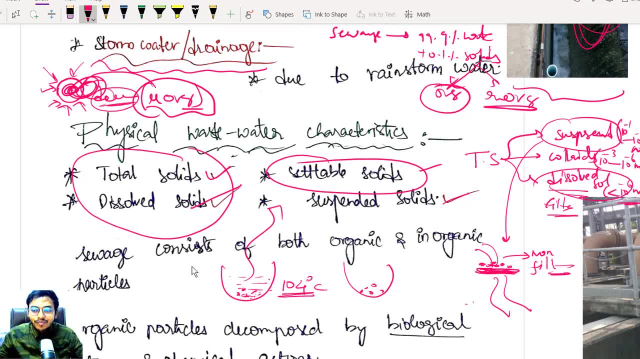 happen, all your water will be evaporated. what is left? only your total solids. weight- this total solids and you will be getting how much total solids are present in your one liter. let us say 10. uh, let us say 100 mg was present. let us say 100 mg of your total solids were present in one liter. okay, 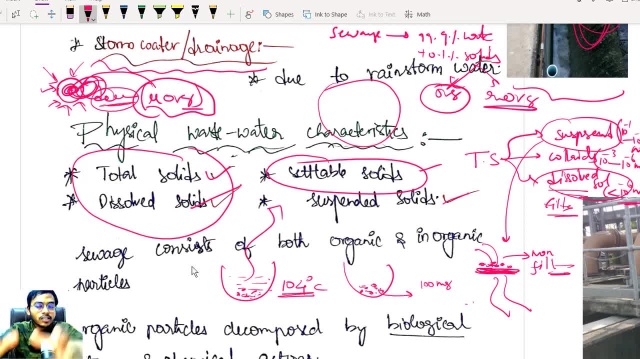 of waste water. you can multiply it and know how much total solids is present in our waste water. agreed or not? okay, now comes the very important question. this is total solids. well and good. what is the component of organic solids and inorganic solids are same concept: drinking water, what you 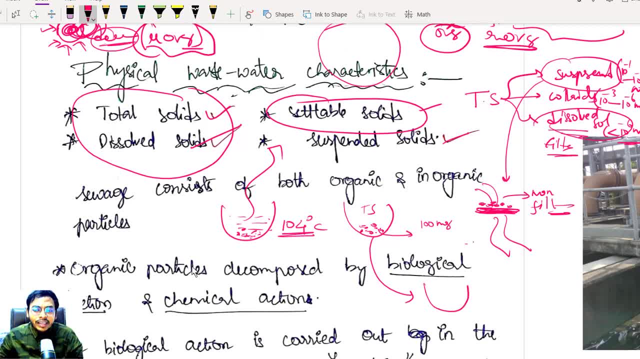 have to do to find organic content or inorganic content. heat this to 600 degrees. heat your total solids to 600 degrees. so when you are heating to 600, right, whatever organic content was present will get completely oxidized and it will be getting vaporized. actually, okay, it will be. 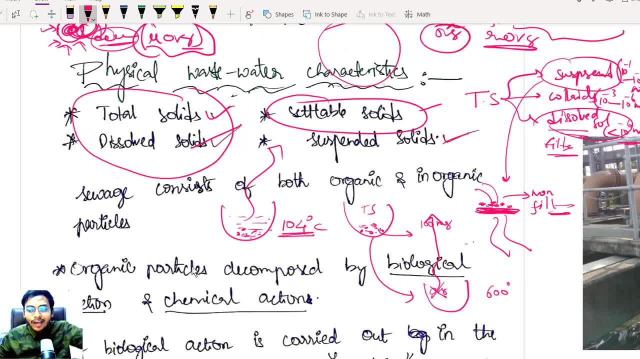 vaporized, okay, it will be completely vanished. so what is left? only inorganic content will be present, okay, so you just wait this. let us say: if total solids is 100 grams weight, this you will be getting inorganic solids. let us say the weight is 60 grams, so 60 milligrams. now what will be the? 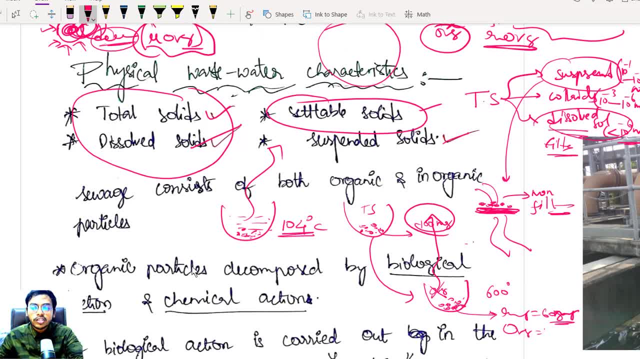 weight of your organic solids. the weight of your organic solids will be 100 minus 60, which will be 40 milligrams. so you have around 40 milligrams of organic content in one liter of water. concept is clear, perfect so far. okay, that is how you can measure your total solids: organic content and inorganic. 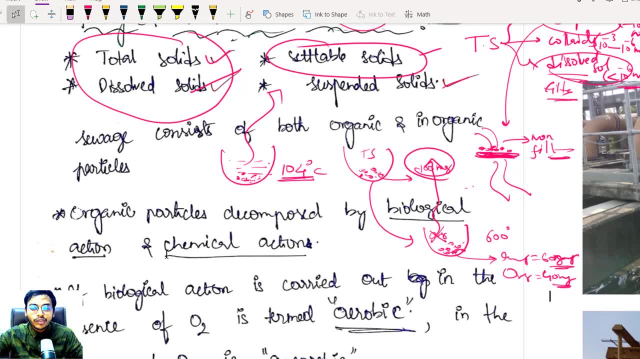 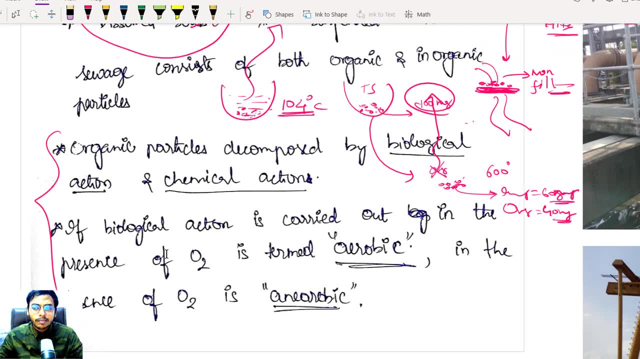 content in your water. okay, now let us continue with this topic and here i have given couple of notes. please make a note: very important bit, especially for small examinations. see, if you are watching this video. there is a high chance you already know this bit. we will study these. 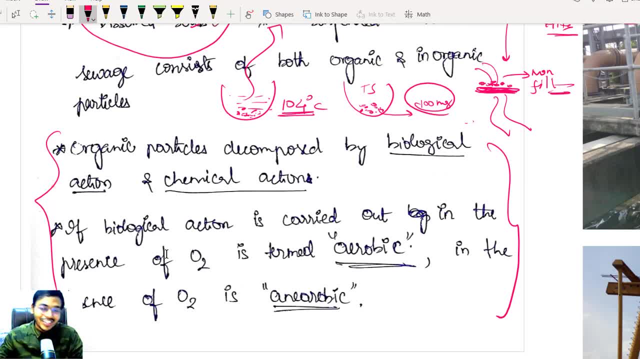 bits in detail also, but let us see here itself. okay, organic particles decomposed by biological action and chemical action. see, i have discussed so far how your organic particles or organic content is being decomposed by microorganisms. right, but we can also decompose it or we can oxidize it using certain chemicals. what are they? we? 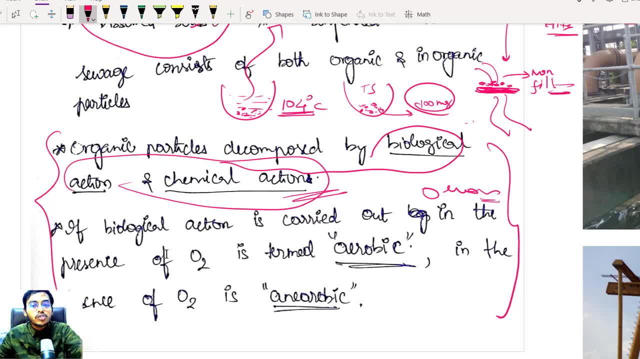 will study it. okay, we'll study it in the next module itself. okay, so our organic matter can be decomposed both by biological action and chemical action. if biological action is being carried out, if this biological action is being carried out with the help of these microorganisms, 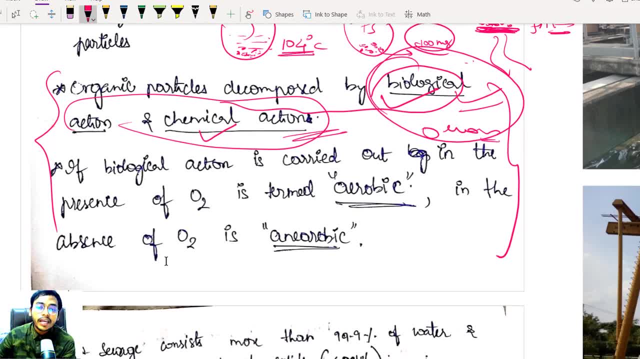 so if your biological action is being carried out in the presence of oxygen, we call it as aerobic degradation or aerobic decomposition. aerobic decomposition if you are doing this in absence. absence means no oxygen. no oxygen is there. if you are performing this biological degradation, we will be calling it as anaerobic anaerobic decomposition. 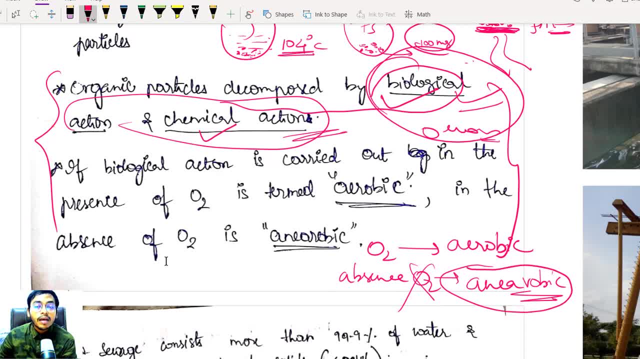 okay, when i am doing this anaerobic decomposition, my end products are very good. i will be getting methane here. i will be getting very stable end products like co2, h2o- not that important- but here instead of co2, i am getting ch4 methane. okay, methane energy produce, therefore, anaerobic is. 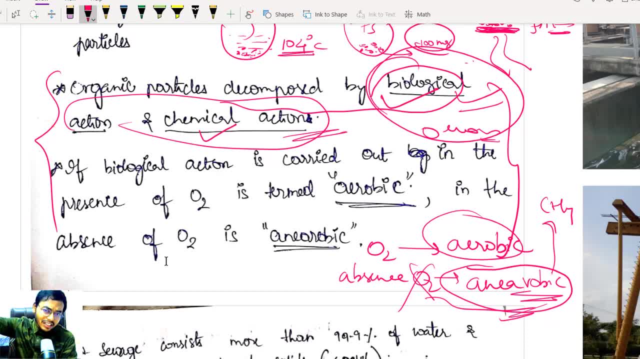 really good. you might ask me, sir, why don't all waste water treatment plants go for anaerobic digestion? okay, because you have to construct anaerobic decomposition. okay, because you have to construct anaerobic in the &y area, but for anaerobic digestion? i will show you. i will show. 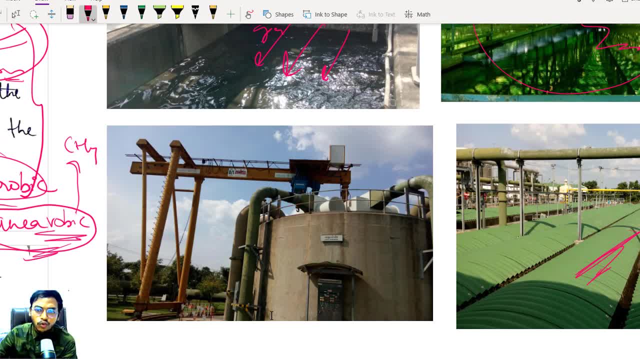 you. this is anaerobic tank which i have seen, uh, somewhere- i don't remember this like four-year-old photo, but definitely not in india. so what happened is: uh, you have to see this much anaerobic tank. you have to construct first of all, if you are doing this for waste water treatment plant, okay, for. 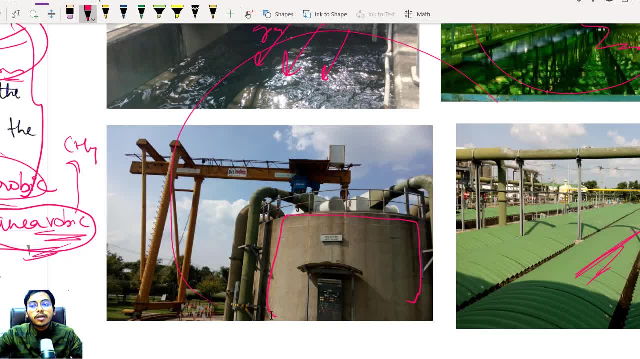 waste water treatment plant. you will be getting so much waste agreed to agrit, so okay, you have to construct such an enormous construction. are getting this point? so more the amount of waste water, bigger your structure will become and it is not economically feasible. so hum na hi jayenge ispe and the energy production from our 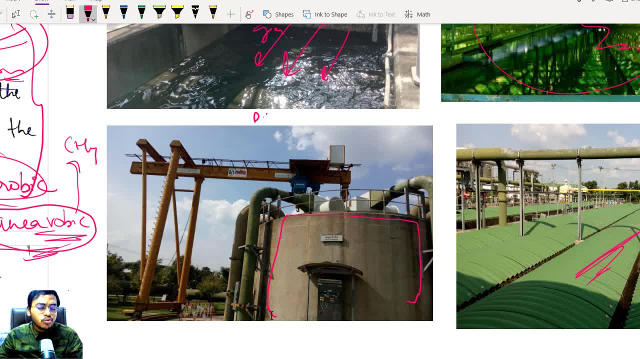 domestic waste water. if from industries, it is a different issue. but if you are going for domestic waste water, right uska organic content na powerful nahi rehta hai. so not that much amount of energy will be produced. but if you have some industrial waste, i am pretty much sure i have taken this. 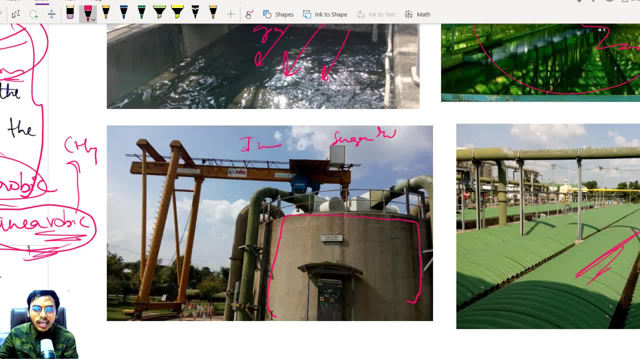 photo: nearby sugar industry. okay, sugar industry, kya aspas liya tha mija yaad nahi hai roughly okay. so, near sugar industry, what happens is at sugar industry you will be using sugar cane right, uska jo bagasse milega okay, molasses jo bhi bache ga. it has high amount of organic content, okay. 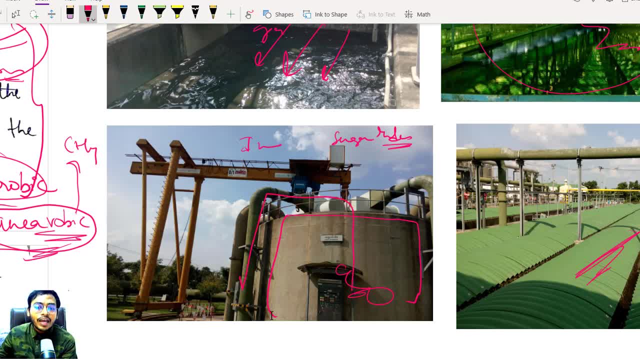 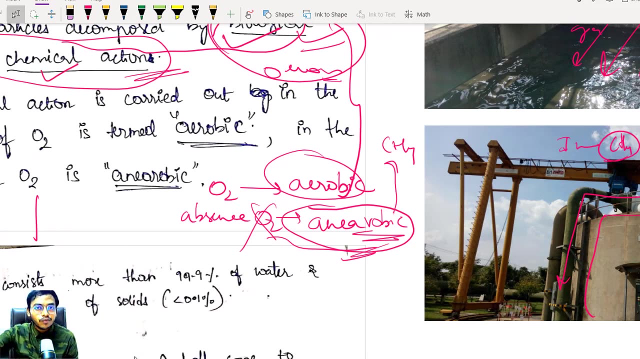 so when you are decomposing it, you will be getting a very high quality of ch4 methane and you will be getting electricity produced because of this methane. okay, aerobic digestion: we don't go almost everywhere. okay, we will be going only at specified places, like industries which deal with food processing or breweries. breweries means- i hope you know right. 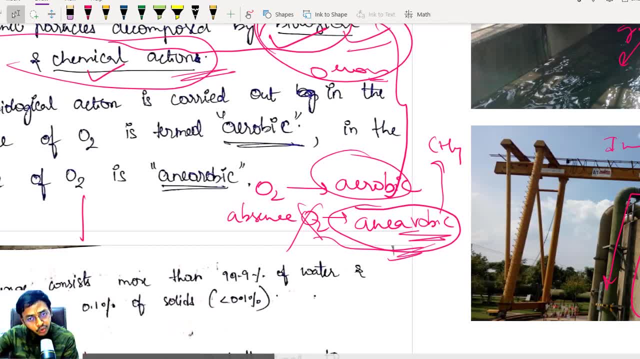 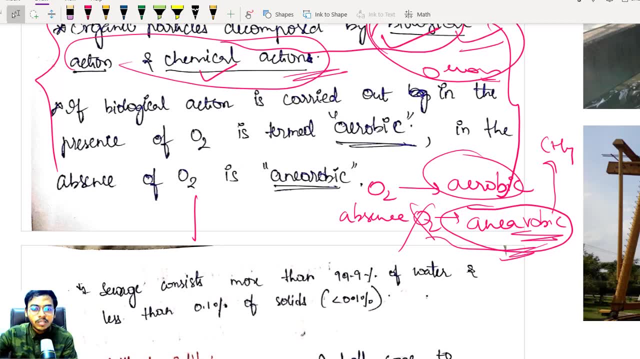 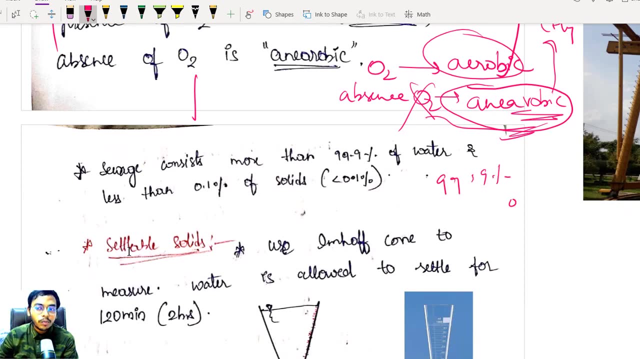 in these areas. basically anaerobic plant will be there. but can you go? yes, of course you can go for domestic also, but economically feasible nahi hota hai. okay, i hope you are getting this point now. this point you already know. sewage consists of: see, in the beginning i have told you 99.9 water and 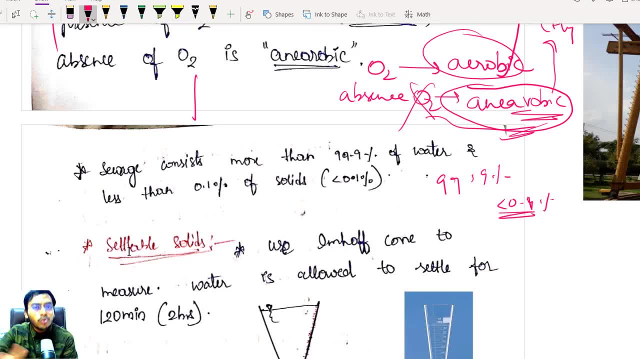 percent solids or less than 0.1 percent solids. it was not fluke. okay, it is a real value. it can be asked in exams also. okay, what is the percentage of solids in our waste water option can be given. it will be 0.01 percent, 0.1 percent, one percent actually. this is a question which was asking. 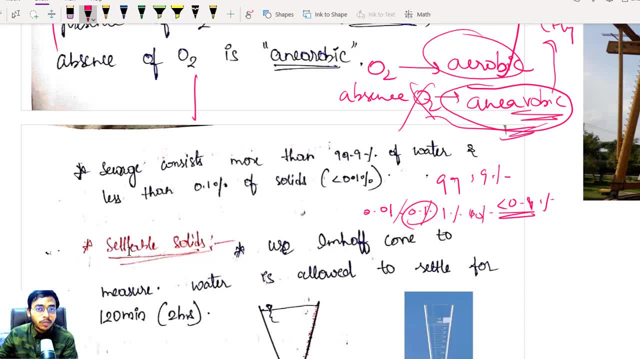 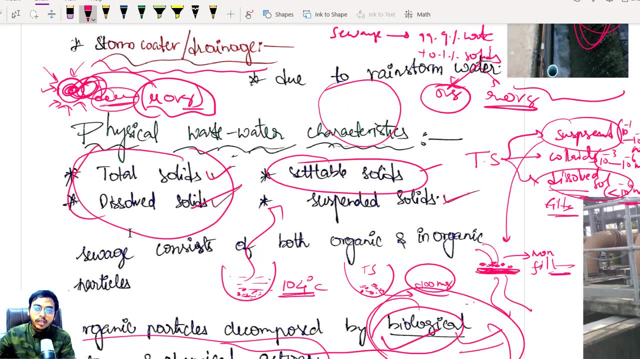 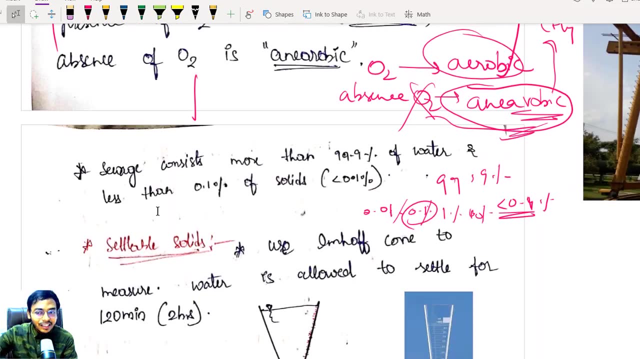 in ssj 10 percent. so what is your option? your option is point one percent, less than point one percent. yadrak lena, okay, see, total solids. you know dissolved solids. you know, you know suspended solids. What is the Settlable solids now, Thomas? Settlable solids, see, obviously in your wastewater you'll. 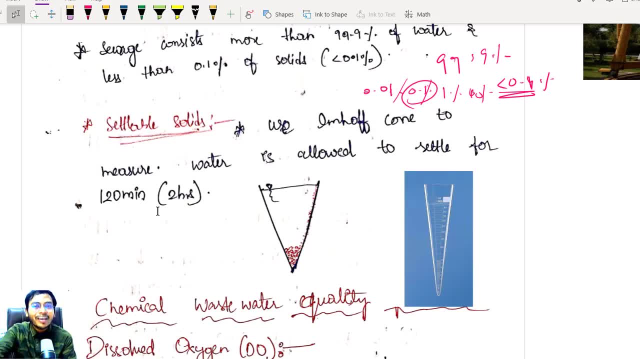 be having little bit of heavy objects right. wastewater a by organic content or Zadar egg- okay, the waste content will be little bit more compared to that of drinking water. So obviously we are getting a new parameter which is called a Settlable solids. what we 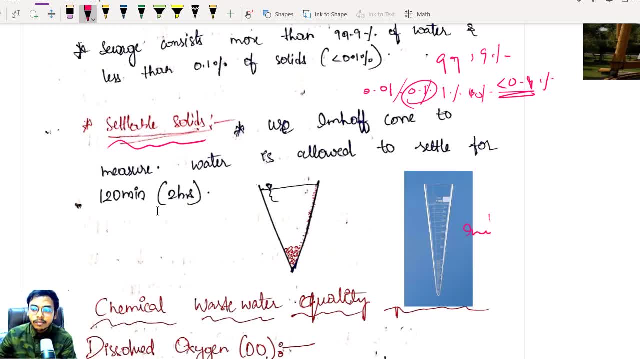 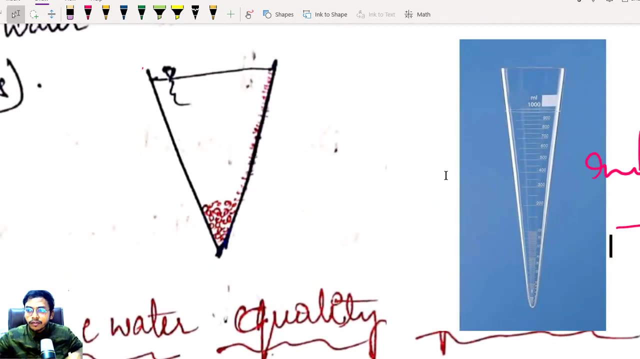 are doing is we are taking him half cone. This is called as him him half cone, So it will be just a triangle on this. if I zoom it, you will be clearly seeing that it is a 1 liter cone. it is a 1 liter cone. can you see it? 1 liter cone in this, you will be. 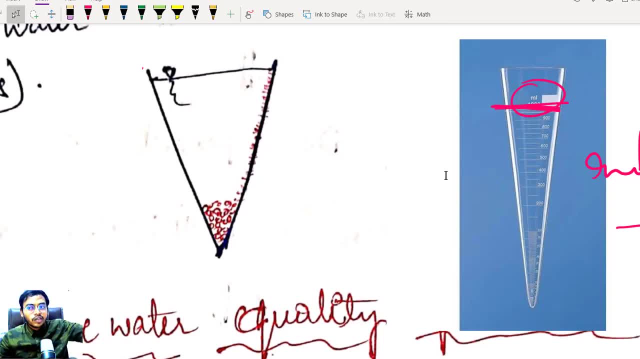 filling wastewater up to this mark. okay, you will be mixing the wastewater well and taking the sample. okay, so job is solid rega. with respect to time, it will be settling down in this coin, agreed, so you will be getting what is the amount of Settlable solids present. 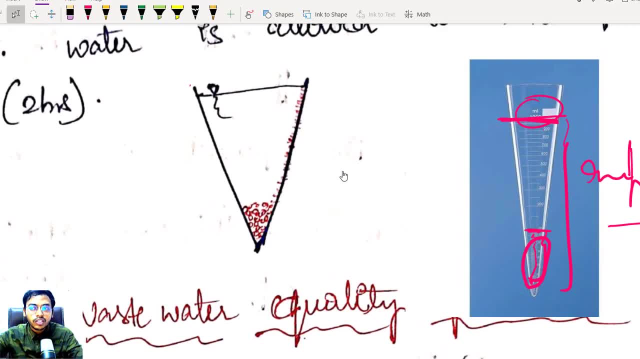 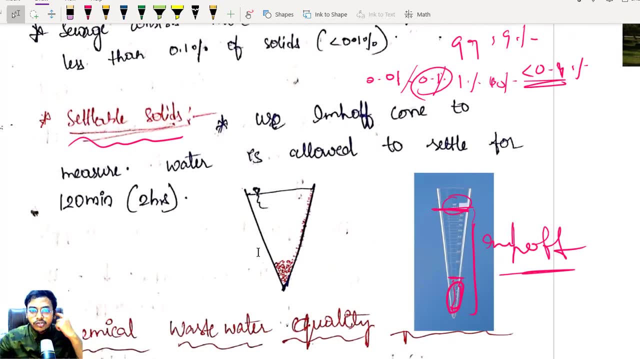 in your wastewater 1 liter solution. okay, in your 1 liter solution. basically, the time which will be given for objects to settle will be 2 hours. that is also one important bit. so what you are using to find out Settlable solids will be using him half cone and water is allowed to settle. 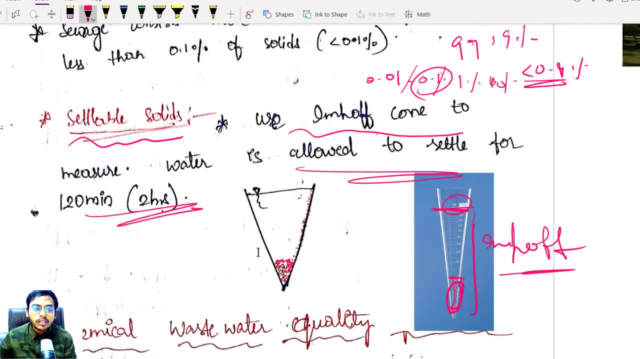 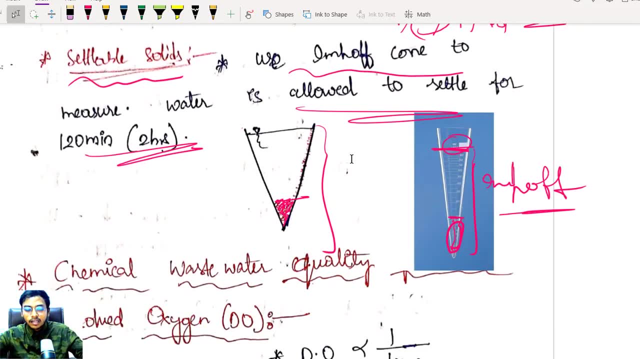 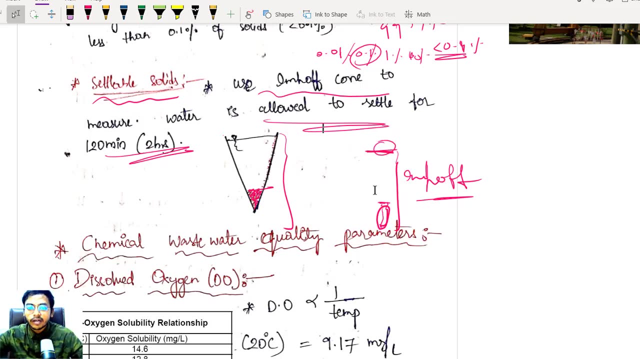 in this him half cone for 120 minutes or 2 hours and we will be measuring how much solids have been settled in this 1 liter solution. okay, I hope concept is clear right now. let us continue with chemical wastewater quality parameters. Let me, let me take this photo out. yeah, chemical wastewater quality parameters. I will teach. 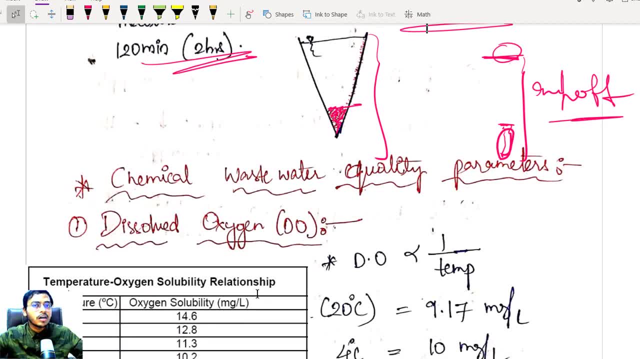 dissolved oxygen and then I will stop. okay, dissolved oxygen. if you understand today, we can understand COD, BOD, THOD, everything in detail. dissolved oxygen is very important. see, it is a very well established fact that most of the living organisms in this world- okay, most, I am saying most, I am not saying every living microorganisms- okay, there are. 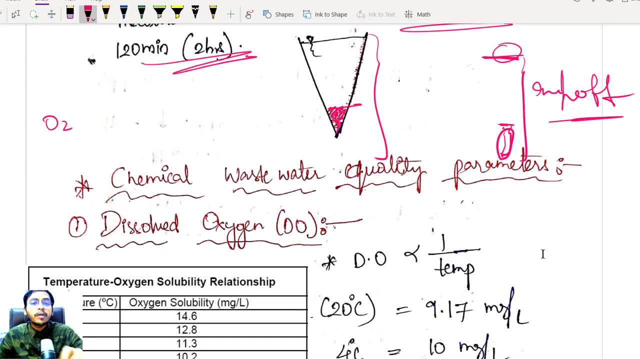 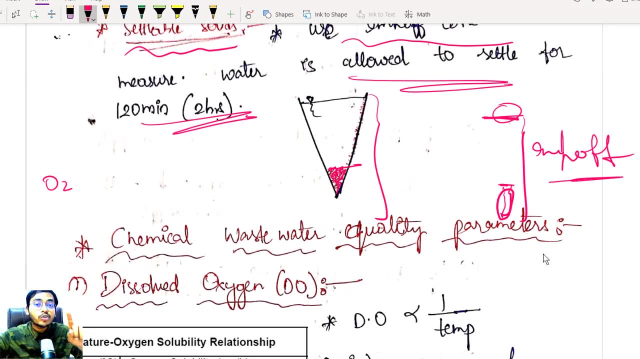 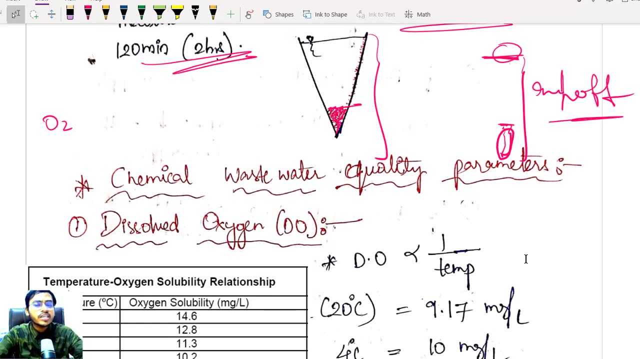 few which can survive without oxygen, also okay. but most they require oxygen for respiration purpose. they require oxygen for metabolism of body and to survive. okay. and aquatic animals are no exception. it can be aquatic plants, it can be fishes, it doesn't matter, they also require oxygen to survive. okay. there are only very few microorganisms which can survive. 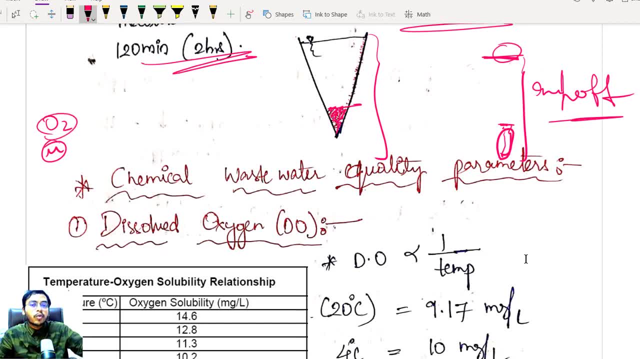 without free oxygen. okay, they are taking oxygen from the bonded form And these microorganisms are responsible for our anaerobic digestion. But these are very rare, These are very few in nature, But most of the living organisms. they require oxygen. Agreed. 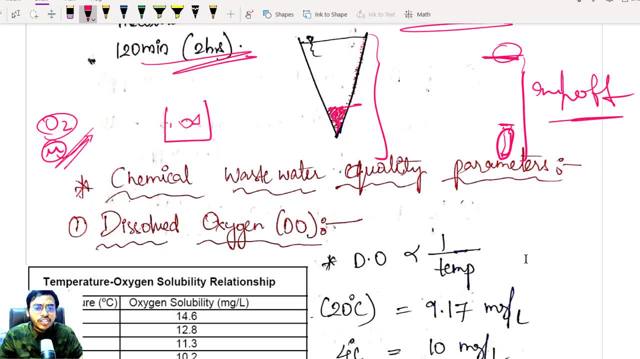 So, in water, these plants or these fishes, how are they surviving, From where they are getting this oxygen? See, the water will have certain amount of solubility. The oxygen, whichever is there, right, It will be dissolved in my water. 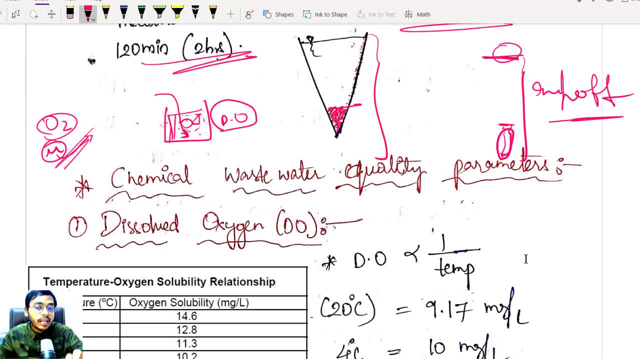 Okay, And this oxygen? I'm calling it as dissolved oxygen And because of this dissolved oxygen, my aquatic life is surviving. I hope concept is clear. And this dissolved oxygen is function of temperature. Remember very important. Okay, It is a function of temperature. 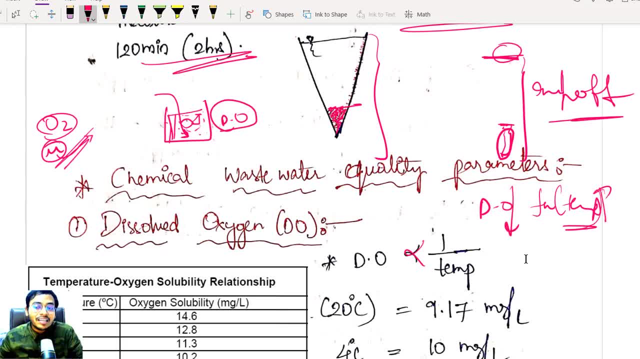 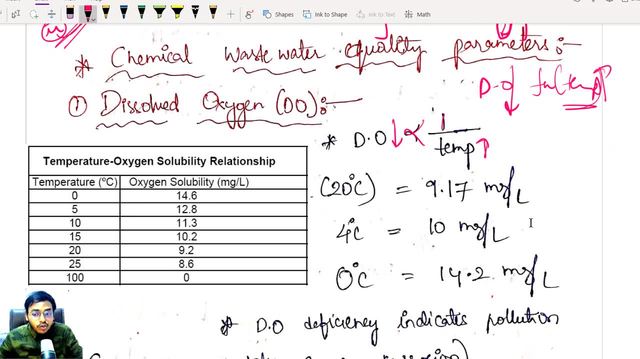 If temperature is more, my dissolved oxygen will be less. They are inversely related. If temperature is more, my dissolved oxygen will be less. And what are the values? Some values you have to remember, At 0 degree centigrade. If there is no pollution, I mean if there is no, uh, any organic substance in water, then my dissolved oxygen at 0 degree centigrade will be 14.2 to 14.6.. Okay, 14.2 to 14.6 mg per liter. 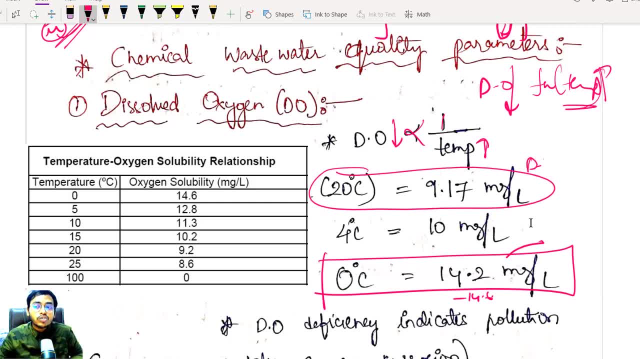 And second most important bit is: at 20 degrees centigrade My DO sat DO saturation or DO without any organic content in that water, My DO will be 9.17 mg per liter, Roughly around 9.2 mg. 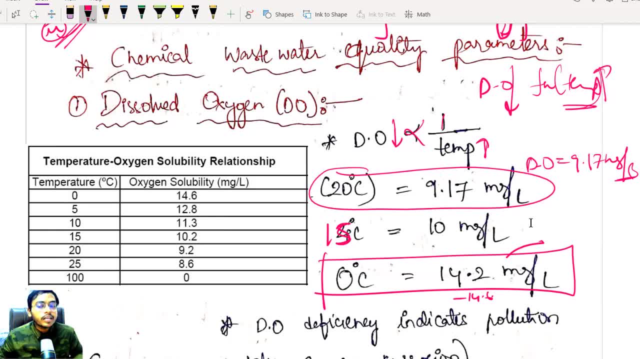 Very important. Okay, Or you can also write for 15 degrees centigrade, because in most of the Western world average temperature is taken as 15 degrees, So 15 degrees is close to 10 at 15 degrees centigrade. 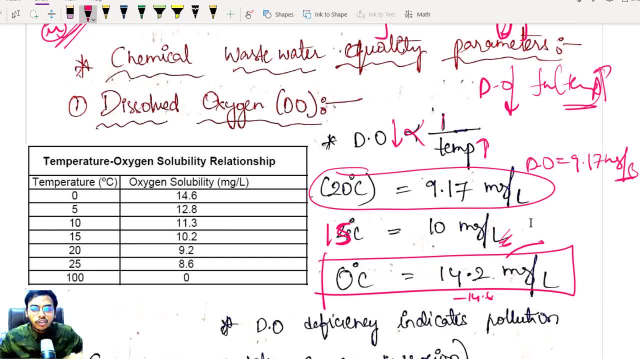 My DO will be around 10 mg per liter. Okay, These three values you have to remember. please do correct notes. I wrote 4 degrees by mistake. It is actually 15 degrees. Okay, You can see the table here. If you want to remember more values, well and good, but for now, remember these three. 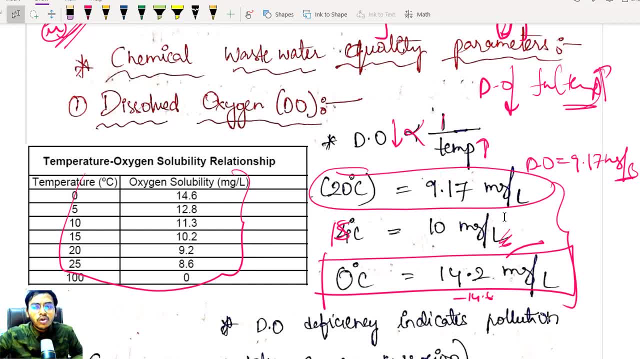 values for objective purpose in examination. Okay, So If there is any value less than 9.17 at 20 degrees centigrade, basically, in India the temperature standard temperature is around 27,. but let us generalize. Let us take some area on which the temperature is around 20 degrees centigrade. 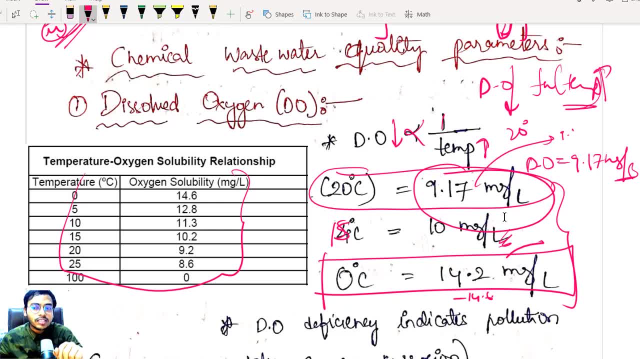 Okay, So you should have a DO of 9.17 in water, but instead of 9.17, if you are seeing something like seven or six, then what does it mean? That means there is some organic content present in our water. 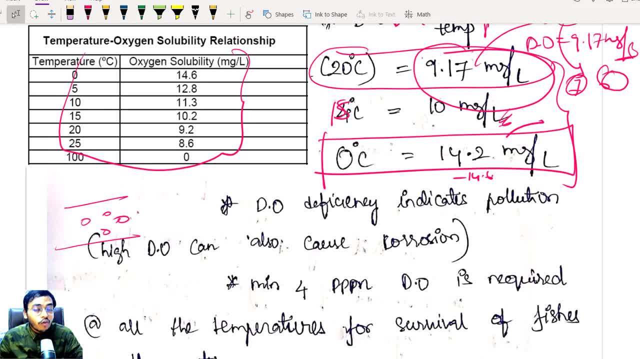 Because of this organic content. what is happening? obviously, organic content should be decomposed. What are the decomposing microorganisms? are decomposing So these microorganisms which are feeding on this food, their food, organic content, So they required oxygen to survey or grid or not. 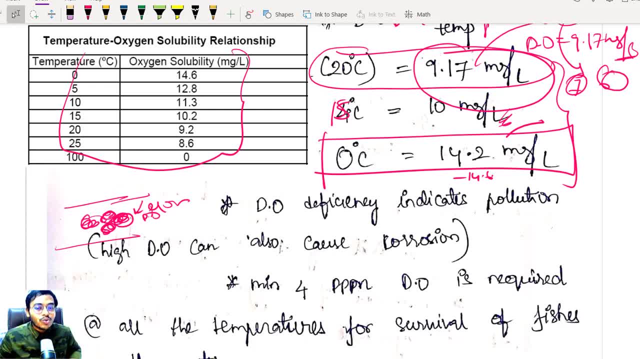 Okay, So they are quickly taking DO from the rest of water. So what is happening? The DO levels in water are failing rapidly. I hope concept is clear, right, Because these microorganisms Okay If they have enough food. I will draw diagrams and show a log growth diagram how the bacteria 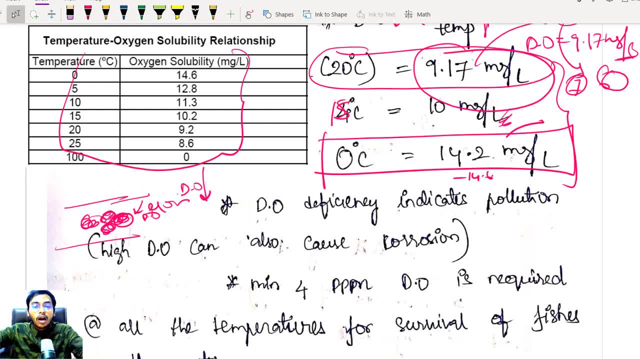 has multiplied itself. So what is happening? Uh, more the organic content, more more bacteria will be produced and faster rate They will be consuming oxygen. Okay, So what is happening? Your DO value will be falling. So if there is any deficiency in DO, that indicates there is pollution. 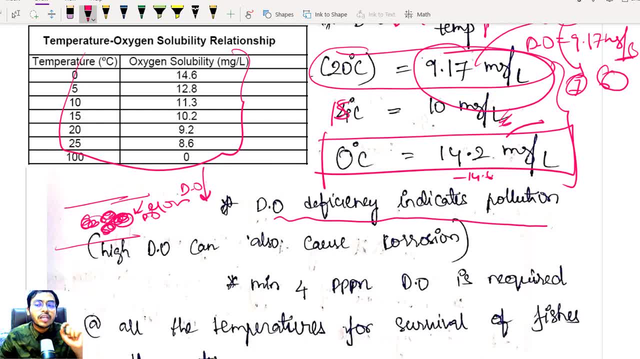 Okay, I hope the concept is clear. Okay, So let us take a look at the next slide. Okay, So let us take a look at the next slide. I hope the concept is clear. right, If there is any deficiency compared to the values which I have just discussed about. 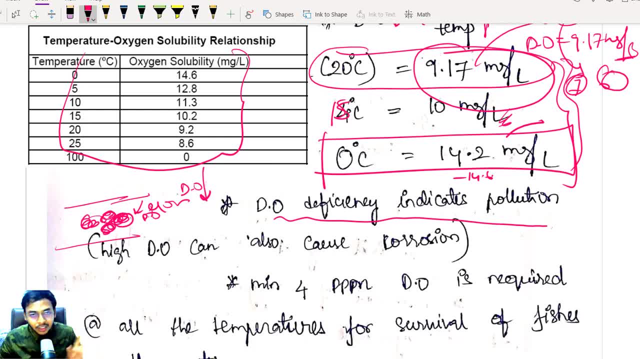 then it definitely indicates that is certain amount of pollution in that water. Okay, If there is less DO, what will happen? Obviously my aquatic life is at risk. If I have high DO, then also it is a problem. I have just given in a bracket. 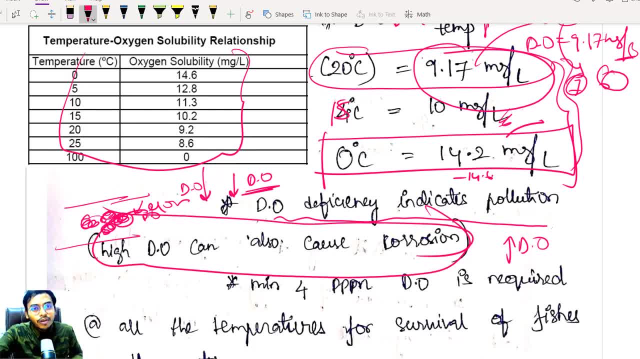 This is not a related concept, but this is a important bit for ESC. Even if you have a high DO, it will be a problem, not for aquatic life. It is good for aquatic life. How much DO you give, It doesn't matter. 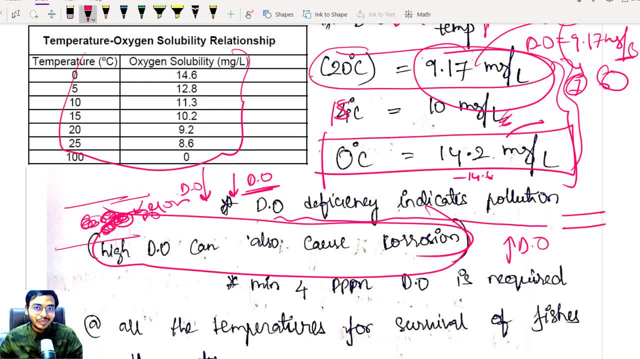 It will be good. But if you are carrying this water- okay, If you're carrying this water in pipes- this DO will be bad because corrosion will happen. What is corrosion? Yeah, If you are taking water in iron pipes, basically we'll be taking cast iron only, right. 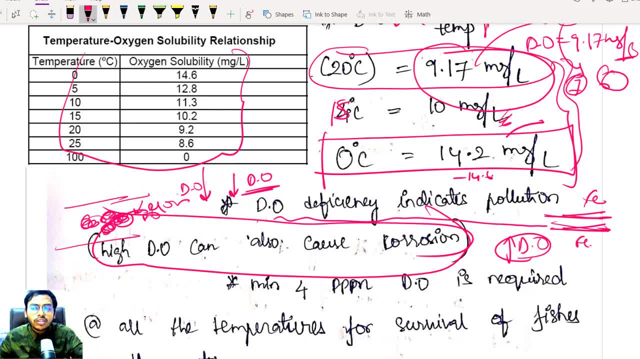 So FE reacts with oxygen and form FE2O3.. FE2O3 is nothing but my corrosion component, right? I hope you're getting this point. So if the DO content is very high, the corrosion can happen in pipes also. This is also one of the reasons. 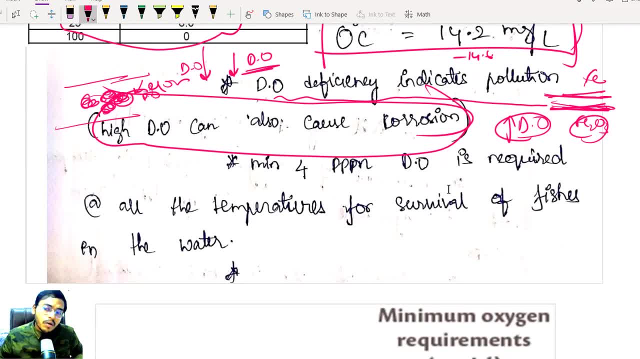 Okay, It can be asked at see how much minimum DO you have to keep so that it will not affect your- uh, it will not affect your aquatic life. That is 4 PPM. 4 PPM, 4 mg per liter. 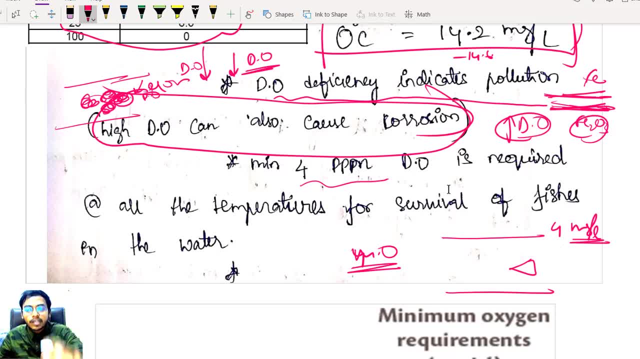 I hope you remember the conversions right. So minimum 4 PPM DO or 4 mg per liter DO is required at all temperatures. whatever temperature, it is Okay At 27 degrees centigrade, let us say around 25 degrees. 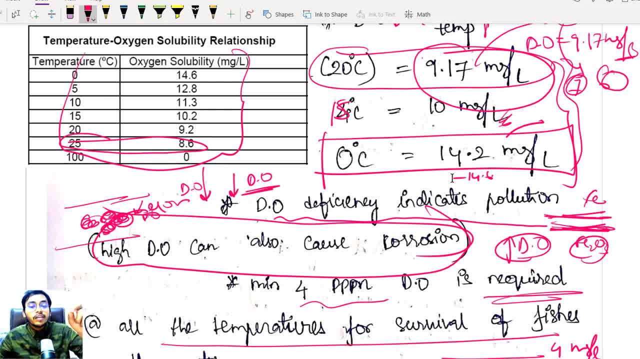 It is already 8.6.. So what is happening If it is falling by any five points? okay, If your DO is falling by five points, less than four, then your aquatic life is at risk. Okay, Your aquatic life is at risk. 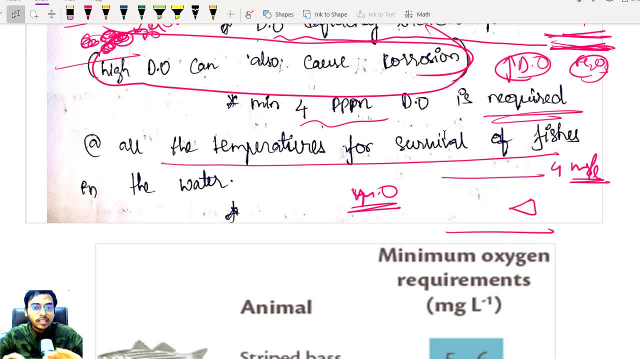 So we have to design our water treatment plants such that in no case my DO will be falling below 4 PPM in water. Okay, Concept is clear. so far, right. I hope you're perfect in DO concept. See, it is not like that. 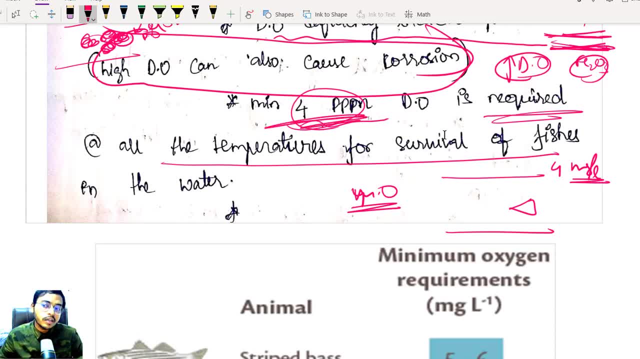 Let us say I have told you minimum 4 PPM should be present. So that might be My fishes and aquatic life will be happily surviving. Not like that, Not exactly like that Many people think. if DO is 4.1, it is safe condition plants and aquatic fishes will survive. 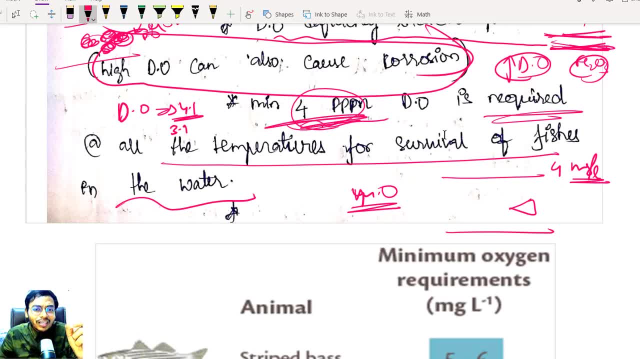 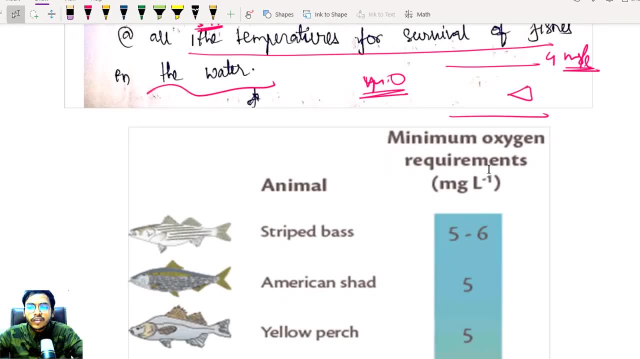 If DO becomes even less than that, Okay, 3.99.. My fishes will die. Rubbish concept, Okay. So I will show you how the effect will be. Obviously, if the more oxygen is there, aquatic life will be happily surviving. 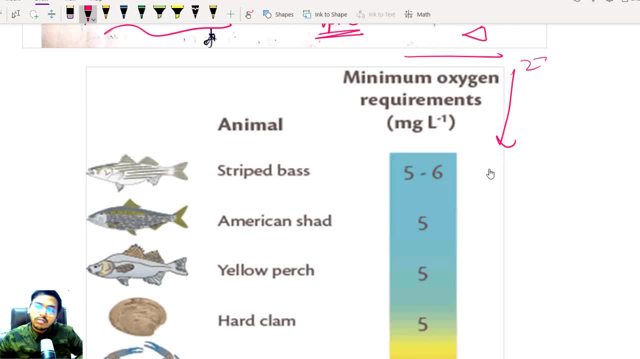 But as my DO value is falling. let us say, at 20 degrees centigrade it should be 9.2 MG per liter, But because of organic content it has fallen to, uh, five or six MG per liter. 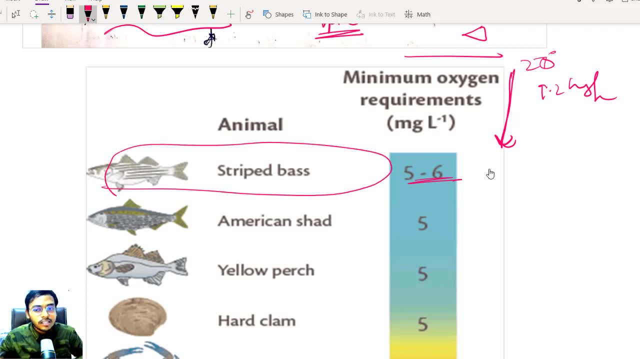 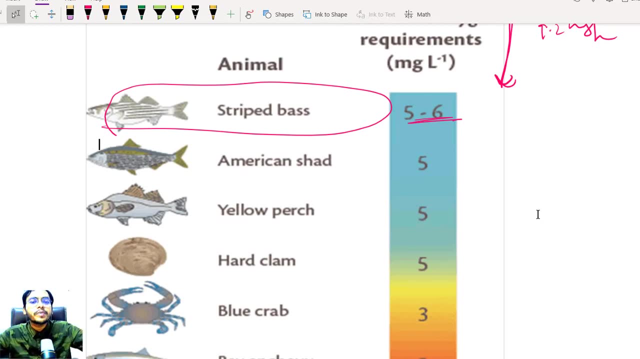 Then what will happen? It will be difficult to find this type of bass type of fishes. Okay, Different fishes required different. There are a lot of fishes, right, There are a lot of species of fishes. different species required different amount of DO levels. 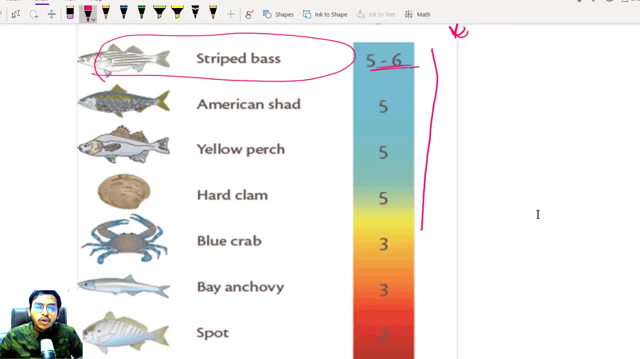 Okay, You can clearly see, as my DO values fall- Falling, these animals will get extinct in that water area. Okay, In that water- nearby water- what is happening? as my DO value is falling, These animals will be getting extinct or, in simple language, they will be dying. 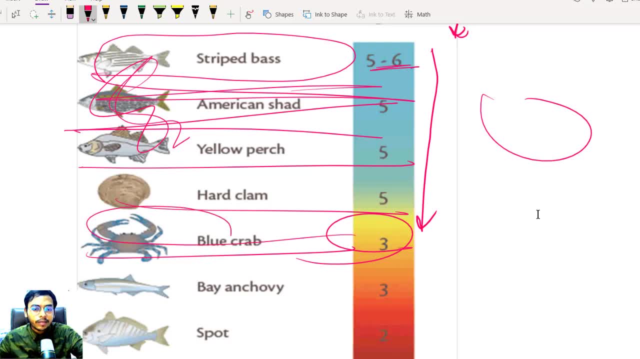 Okay, They will be dying. If DO is falling below three, my crab will be dying, and so on. But most of the fishes right. They can survive at 4 PPM, 4 PPM. That's why we are taking this value. 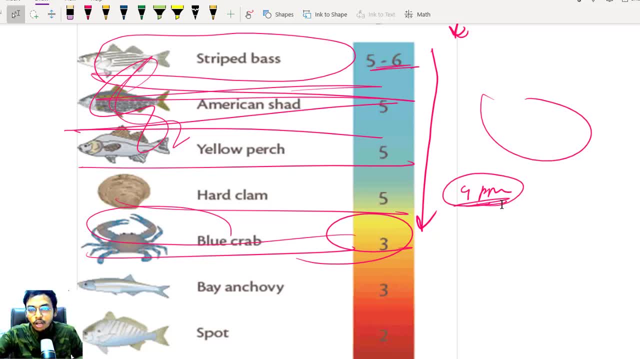 Okay, It doesn't mean Just to above that All my aquatic life is safe And just Below it, all my aquatic life in danger. It doesn't mean like that. Okay, You can clearly see that, as my DO is falling. these all species go on extinction. 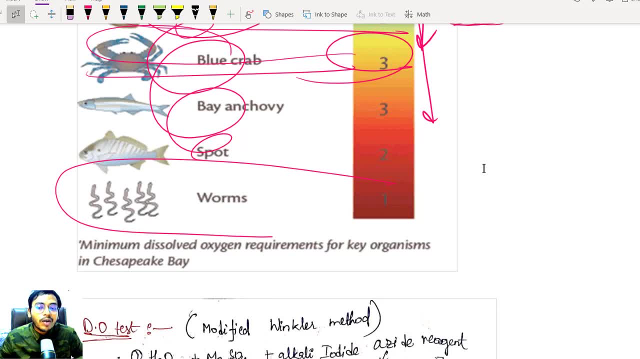 Okay. So even at a DO is close to one, there might be some worms surviving here. Okay, There might be still some worms surviving. Okay, I hope you're getting this point clearly Right. Even if DO is falling to that level, there might be some life, but majority of life will be gone. 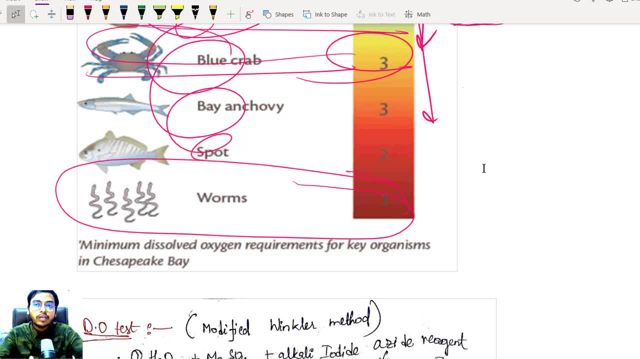 That's why we are taking the minimum value for DO as 4 mg per liter. If you're allowing anything less, Then definitely our environment is at risk. Okay, Most of the animals, most of the animals- lies in this zone of three to five. 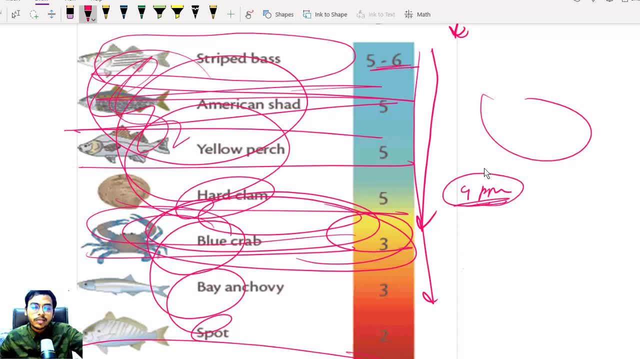 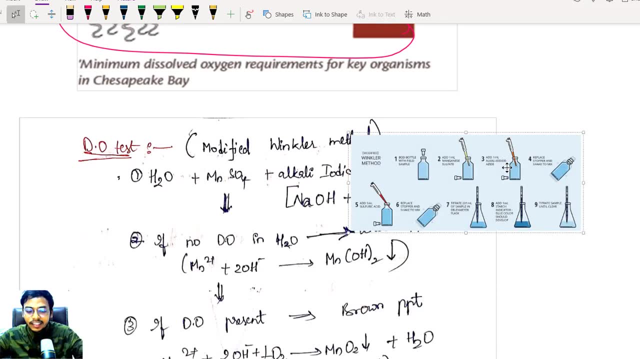 Okay, If you are falling below four, definitely most of the species will be at danger. Now let us see how to calculate this DO value, and then I will stop. Okay, Let us directly see this test so that it will be perfect. 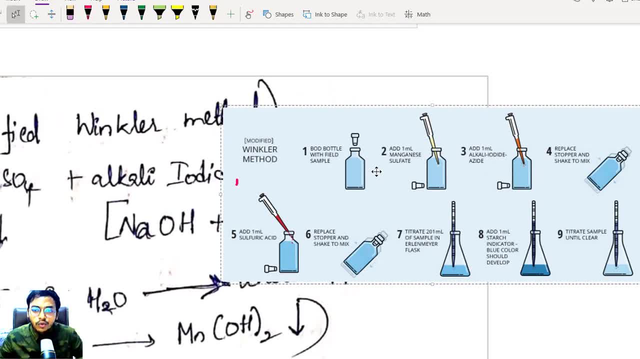 The test which I'm calling for to finding this DO right. That will be Winkler's method or Winkler's test. So first you will be taking BOD bottle. See what is BOD I will take. I'll teach you in the next model. but BOD bottle generally it will be 300 ml. 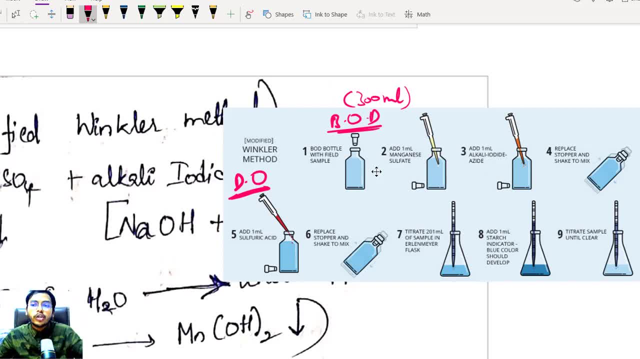 You take that BOD bottle, Okay, And this. what you have to add is manganese sulfate M N, manganese sulfate SO4.. Okay, Just add manganese sulfate. So now this is nothing but water, wastewater, whichever you are having. plus manganese sulfate, plus manganese sulfate. 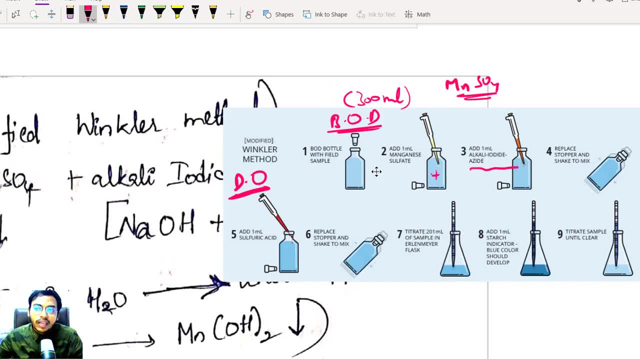 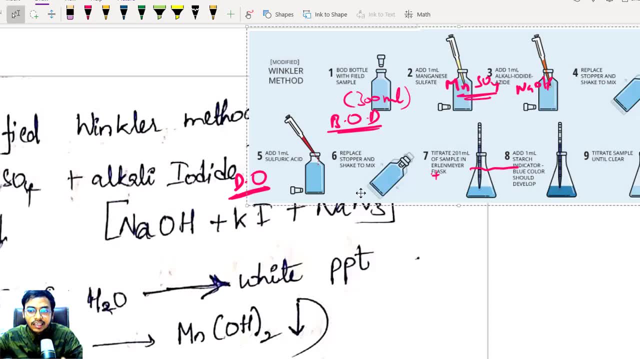 Now to this, add alkali iodide aside. Okay, When I'm talking about alkali, what is it? It is nothing but NaOH. See, You need not write the notes, Everything is clearly given. You can clearly see that NaOH. 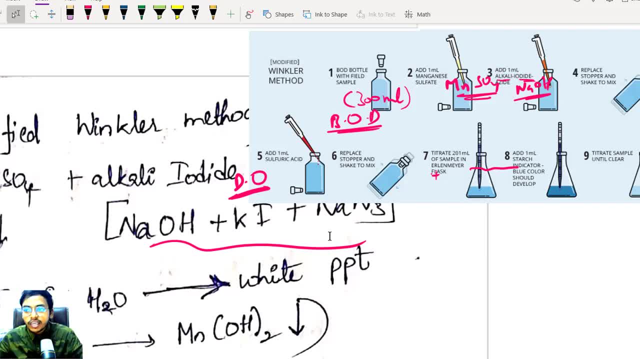 So alkali is NaOH Iodide. I'm talking about potassium iodide. So plus Ki. And what is this azide? Azide is NaN3. Azide is NaN3. So this is called as my alkali iodide. 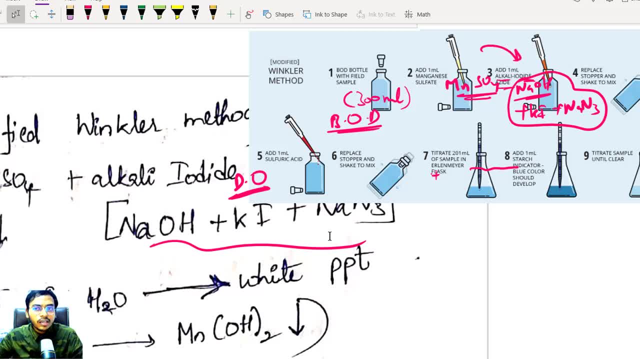 I said: I'm adding that to my manganese sulfate solution. Okay, Manganese sulfate, Remember this term very important. And then what you have to do: You have to shake it. You have to shake it properly. Now comes the very important statement which I have already made here. 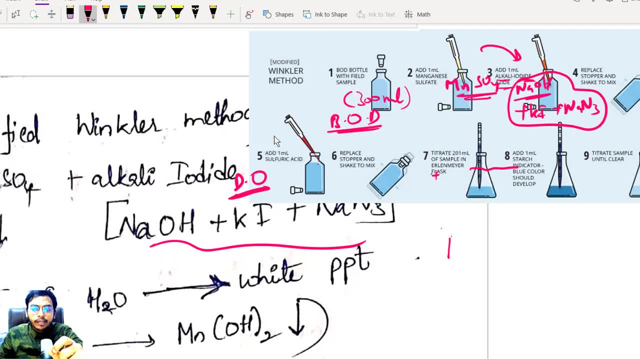 See after you shake, right, If there is any white PPT in your bottle, okay, if this is my bottle, 300 mm bottle, whatever- sorry, but I hope you are getting it right. It is my POD bottle, Okay. 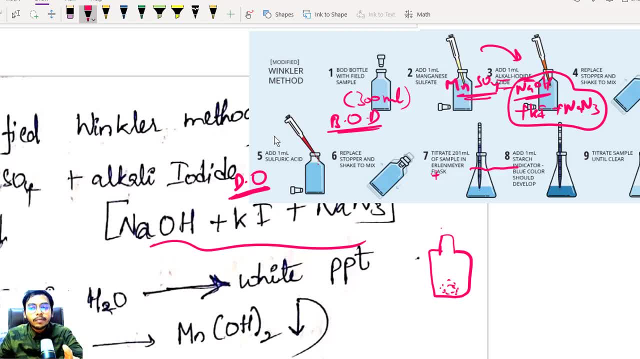 If you are seeing white PPT formate right, Then that means all your dissolved oxygen is gone. The DO value in this soil sample is zero. Just write zero. Your experiment is complete. Your experiment is finished. but instead of white, if you are getting brown PPT, then that means there is some DO. 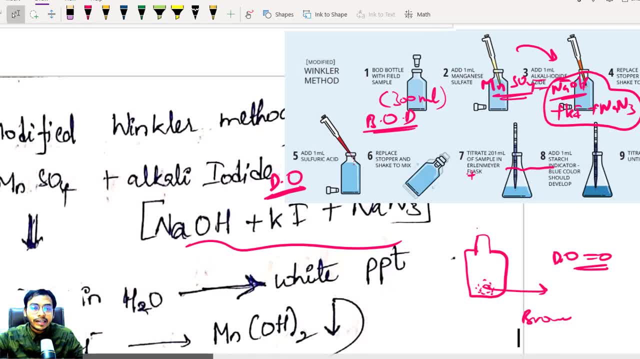 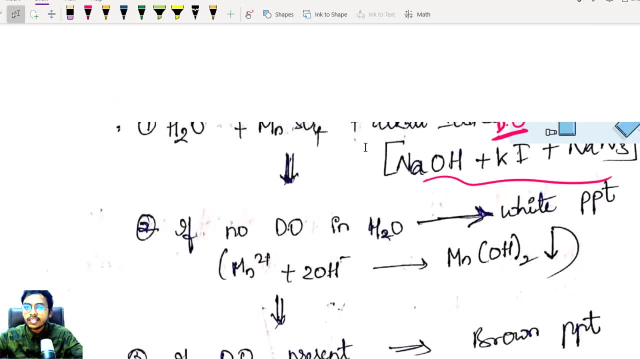 Why I will show you why I will show you. see this manganese right, It requires oxygen. It reacts very quickly with oxygen. So when I'm having this manganese sulfate, when I'm having this manganese sulfate, let me show you. let me show you this equation. 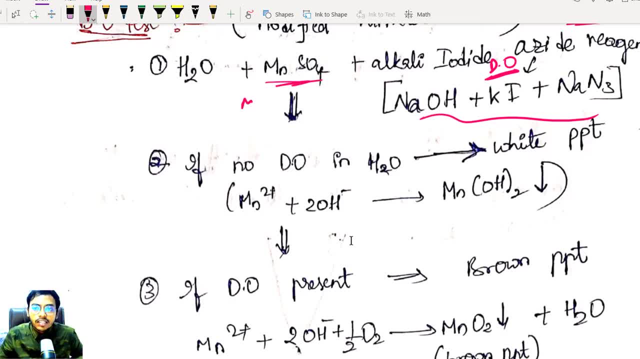 Yeah, So when I'm having this manganese sulfate, which is nothing but MN2 plus, it will react better with oxygen. So is there any free oxygen Here: H2O plus MNSO4 plus alkali iodide acid reaction. 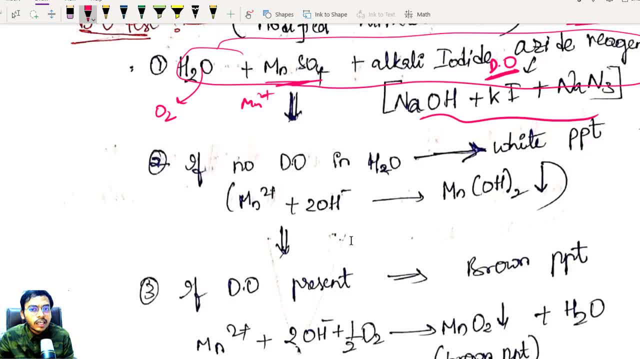 Okay, So there is no O2, right? If this water doesn't have any dissolved oxygen, then it cannot react with oxygen. So what it will react? it will react with OH only. Okay, So MN2 plus plus 2OH, what you'll be getting? MNOH taken twice. MNOH taken twice manganese hydroxide. 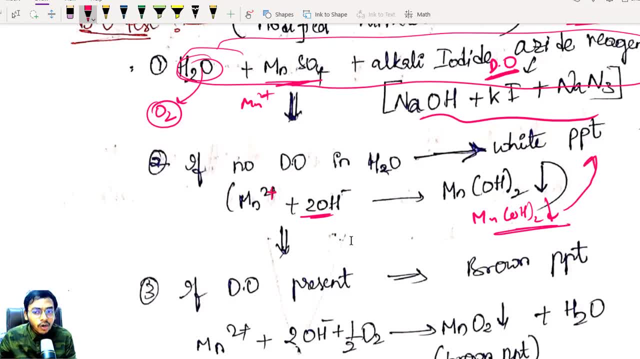 This manganese hydroxide is a white PPT because it is forming. It means there is no oxygen. Therefore, You are getting white PPT. What will be your DO value? DO value is just straight forward. You have to write. it is zero. 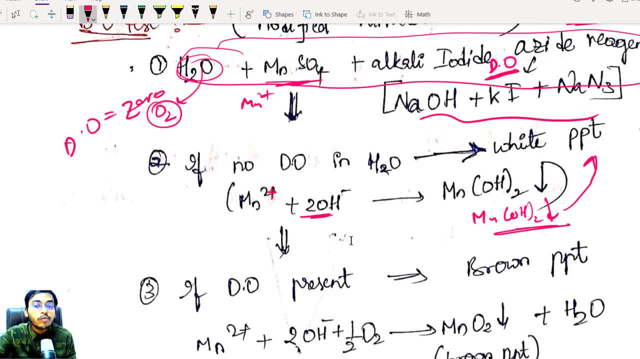 Okay. Instead, if it is forming brown PPT, that means there is some oxygen. What is happening? Let us try to understand. if in this water, if in this wastewater, if any DO is left, then what will happen? Obviously, my MN2 plus. it will react with this oxygen. 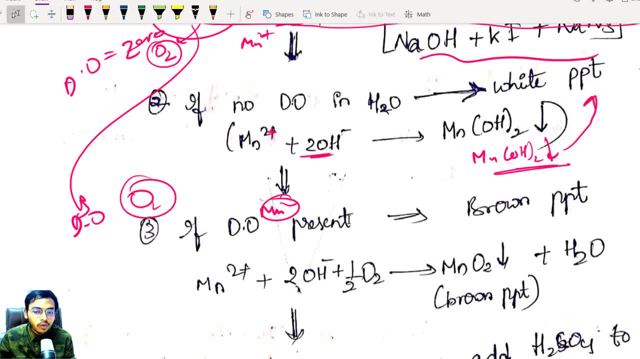 Okay, It will react with oxygen which is present in water, So MN2 plus plus 2OH minus plus half O2.. It will be reacting with oxygen and I'm getting MN2, manganese dioxide. This manganese dioxide is in brown color. 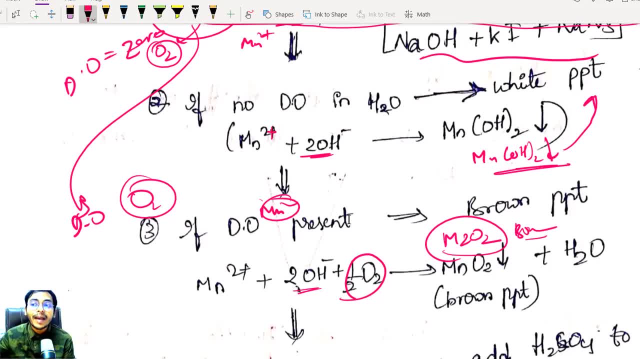 Okay, Is in brown color. A bit can be formed. What is the color of manganese hydroxide? option is white. Okay, Right Option is white. And what is the color of manganese dioxide? Answer is brown. Okay, If the manganese dioxide is formed, that means it has reacted with oxygen. 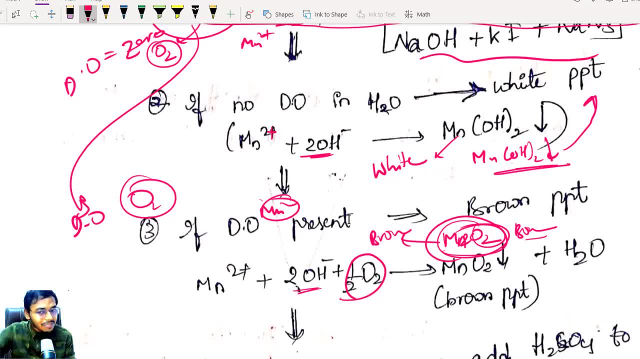 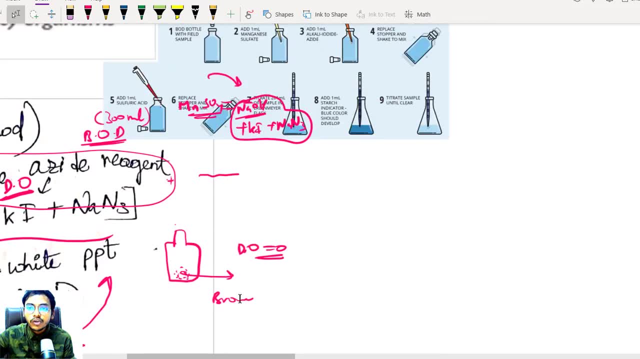 Right, That means free oxygen is available in water That is dissolved. oxygen is present in my water. Now, What You have To do is now what you have to do if you are getting brown precipitate in your diagram, sorry, in your experiment. if you are getting brown precipitate, then go for further methods. 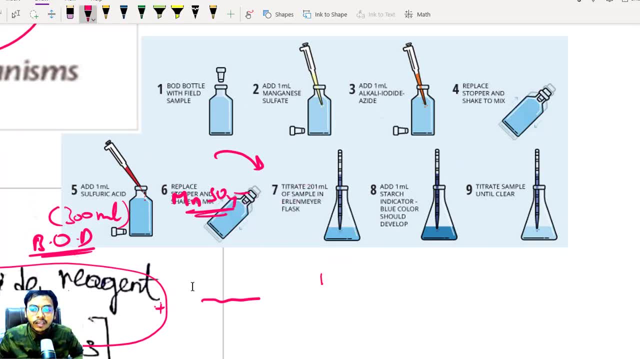 to find DO value. Okay, Or else your DO value. white PPT experiment is finished. White PPT experiment is finished. Your DO value is zero. If brown PPT continues the experiment to find what is your DO value. how to find? very simple. 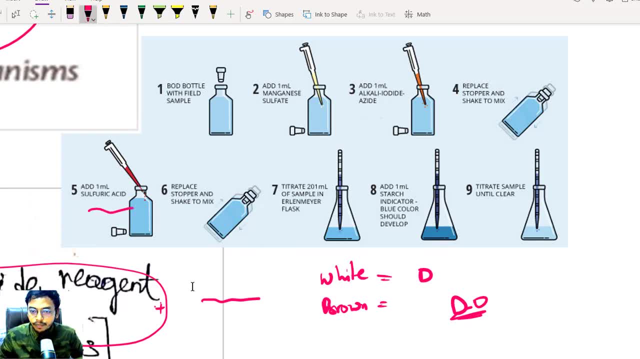 that just add one ml sulfuric acid to it. What are you adding? You are adding H2SO4.. See When you are adding H2SO4, acidic media: see here you have alkali in alkaline medium. The PPT was formed. 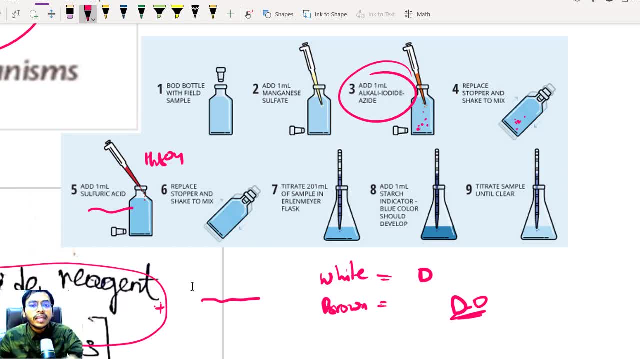 The PPT was formed. Precipitation was formed. So when you are adding acid to it, what will happen to the precipitate? It will again get dissolved. Common sense ki baat hai, Okay. In alkaline medium, precipitate was formed. 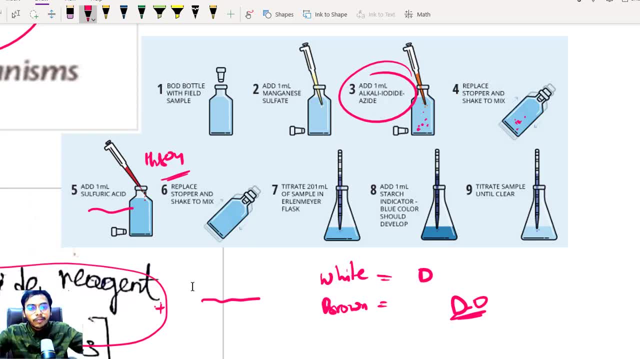 Add acid, acidic medium, ho jayega. So whatever precipitate was formed, it will be dissolving again. Okay, So you are. whatever brown precipitate was there, right, It will be dissolved in water. Now again, You shake it very well. 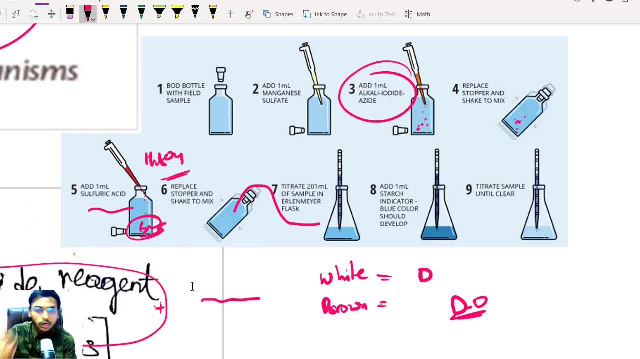 Okay, After shaking it, take this, uh, take this, whatever water. right, You are waste water into such flask and add one ml of starch indicator to it. Okay, What are you adding? You are adding starch indicator to it. 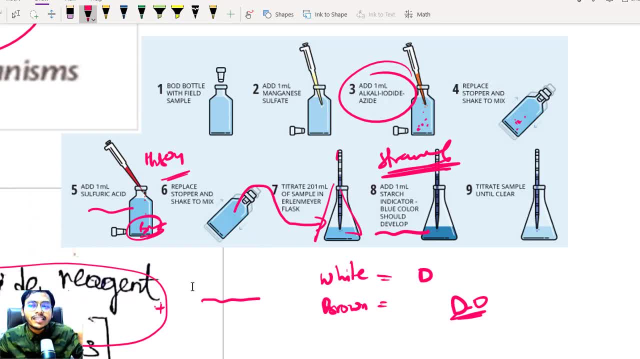 So I hope you know this right, Chote, jab se padte aa rahe ho starch indicator, jab bhi add karte ho, toh water kunsa color ho jayega. blue color ho jayega. Okay, So now your waste water is in blue color. 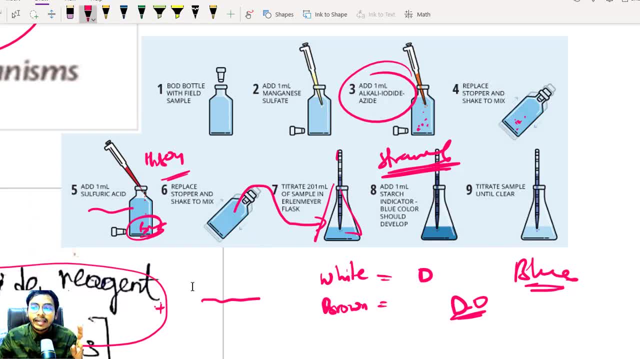 I hope you are getting this point Now. titrate it. Now. titrate it with sodium thiosulfate, Sodium Na2H2O3, sodium thiosulfate se titrate karna. So when you are titrating, the color change will be from dark blue to light, uh, to clear color or white color. 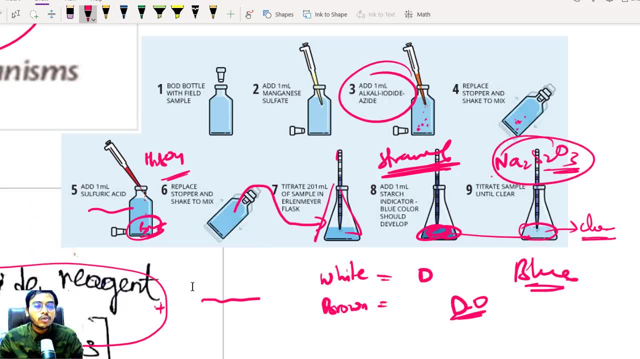 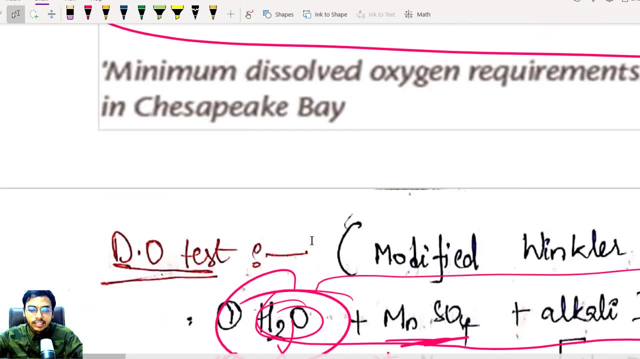 Then we'll be stopping this experiment. Okay, Based on this titration value, you can calculate and find out what is your DO. as simple as that. Okay, As simple as that. Let us see whatever I have given here. Let us see the text one, and then I will stop. 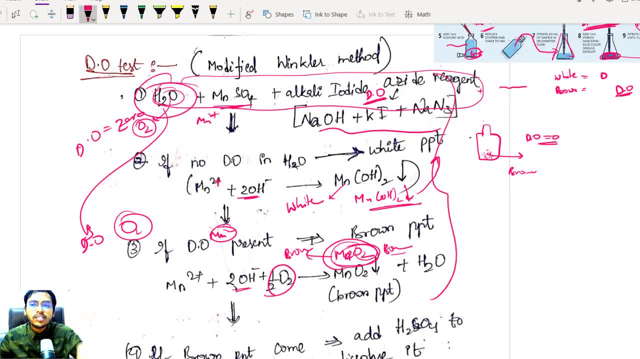 So so far you are clear, right. So what is the test? Very simple. What is this Winkler method step can directly ask in examination: take your waste water, add manganese sulfate, MN, SO4, and alkali iodide azide. 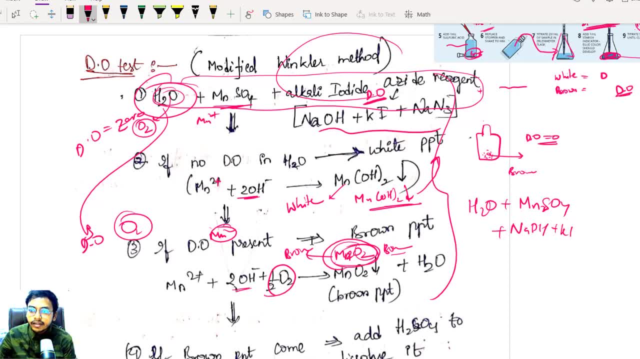 Alkali iodide azide is NaOH plus Ki plus NaN3, plus NaN3.. So now my solution is ready. If it is giving me white precipitation, DO value is zero. DO value is zero. If it is giving brown precipitation only, then you have to add H2SO4.